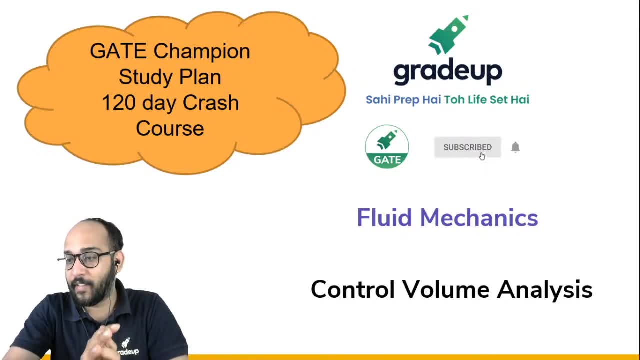 Once again, welcome back. Hello, Jeevan, Very good evening. How are you all Fit and fine? Very good evening, Vineet Hi Rajesh. Very good evening. So, guys, come on, join in quickly and also do share the information of this session with your friends. 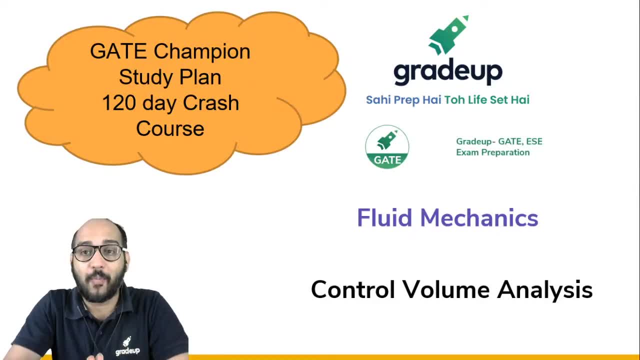 as well. Okay, so the content is. I hope you like it. It is free of cost, so please share it So that more and more people can join and they can also get benefit. Now some quality questions that we will be solving today on control volume analysis. 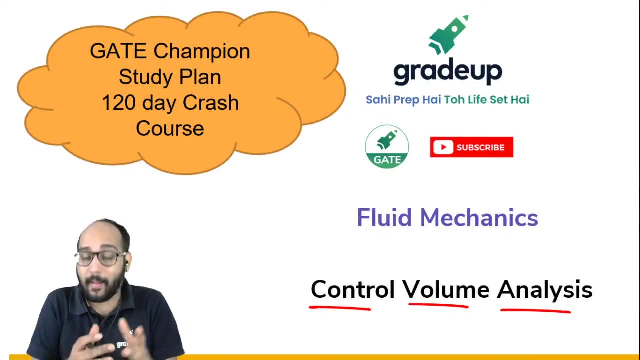 So, basically, we will have a mixture of questions today. We'll be starting off with impulse momentum principle. If you have ever had this doubt, sir, when to take plus minus directions and all those. everything will be clear today And also after doing some analysis of that. 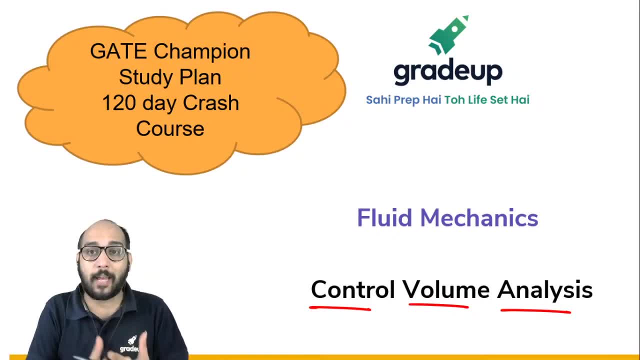 question. we'll be moving on to some very interesting miscellaneous type of questions that were already asked, along with a very special case which is very, very important as far as the great examination is considered. Once it was asked, but it was expected for. 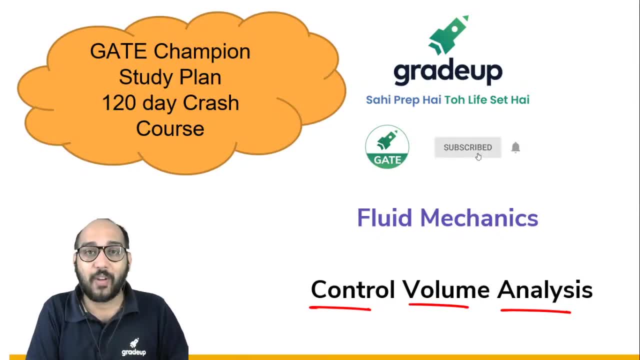 a very long time. You never know, 2022 is that lucky year, Okay. So we'll be talking about all these in this particular session. So for topics, you guys do share the session And if you like it, you would Bestly like button as well as share this session. Okay. 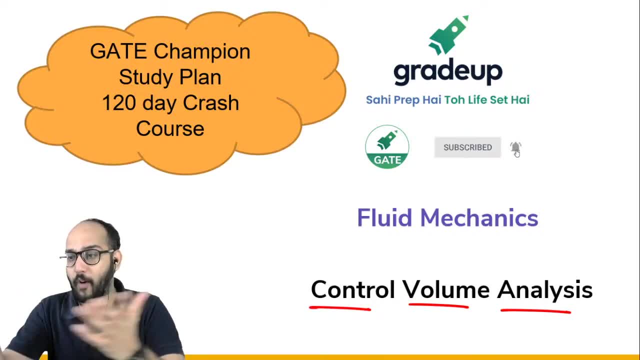 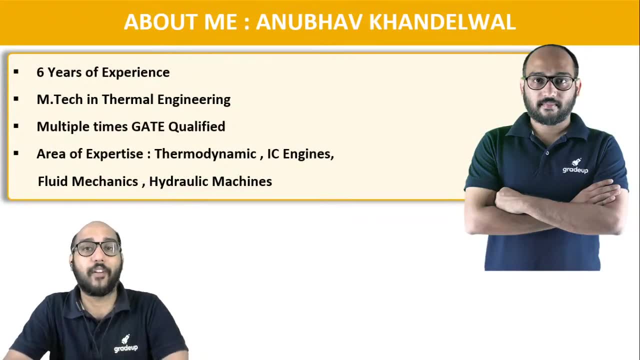 so us start, guys. very good evening. i guess many of you have joined in, so let us start with this session. so anyone who has joined in for the first time, just a brief introduction about myself. my name is anwar khandelwal. i have a little more than six years of an experience in this field. 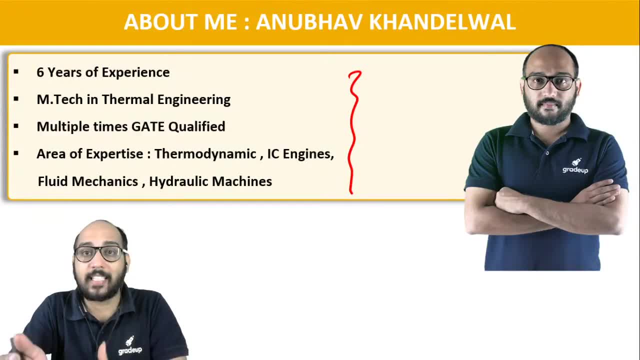 where i try to help you out guys, whether it is gate, esc or any other psu exams, to help you out, to guide you, to make sure that you are always on the right track. okay, i've qualified some of the examinations, like gate as well as esc, and normally you would find me discussing topics on subjects. 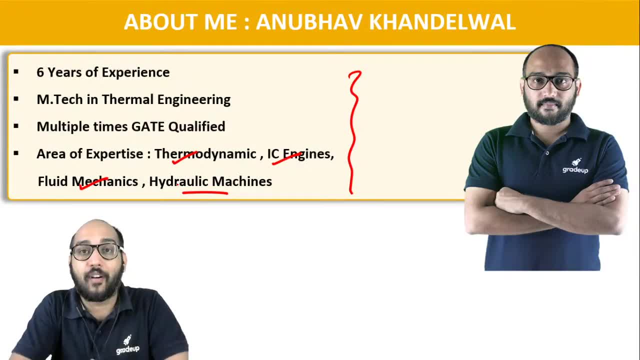 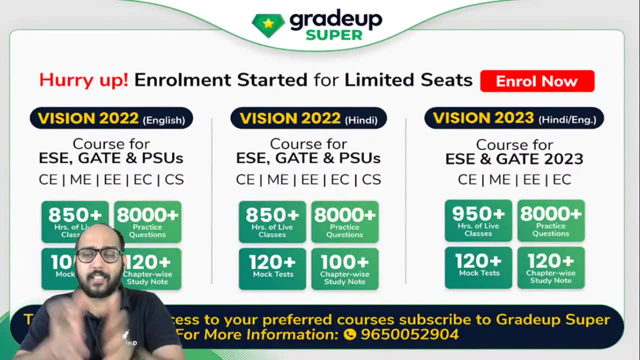 like thermodynamics, ic engines, applied fluids as well as hydraulic machines. okay, so, let us uh start. before that, just a brief about what we have as an offer to you in our vision batches. so if you are preparing for esc, gate psu, which means all of the examinations so that for this we have our 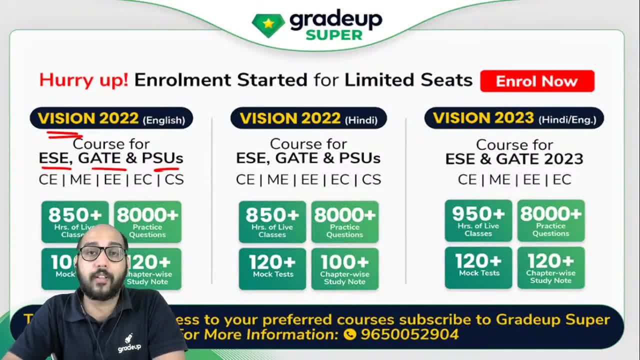 vision batch. so enrollment is open for these vision batches for both 2022 as well as 2023. you want to study in hindi? there's a batch. you want to study in english? there's still a batch for that. okay, so you demand your requirements. we are there to help you out. then our live classes. we discuss lot of concepts. 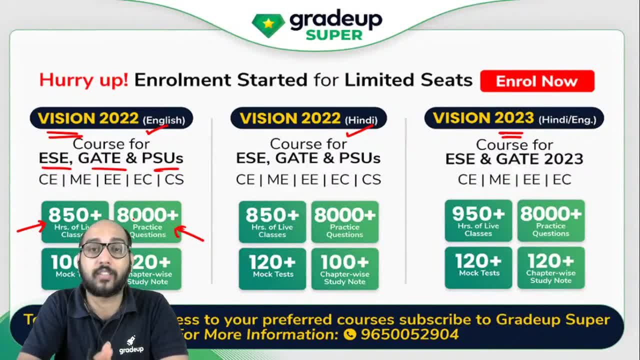 also practice questions, not only in classes, but as well as in the form of quizzes. you get notes as well as access to a lot of mock tests. so for this you have to have a great up super subscription, and this is the number at which you can call for further details. okay, so people have joined in. okay, so those who have joined in those. 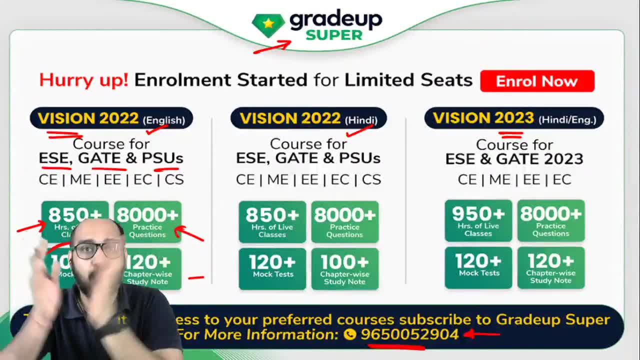 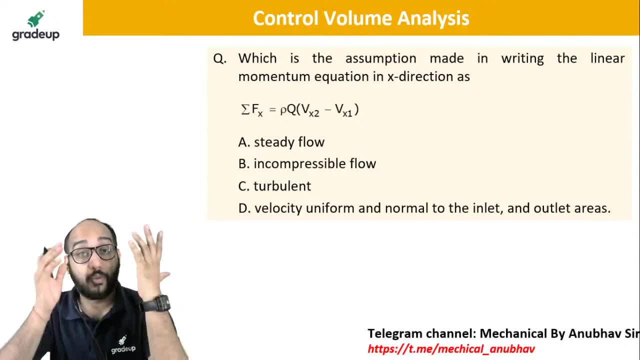 who are still there first, that's what. but out live view to jada hona to address you some very quality questions. people should be there, and also those who are joining it. just a humble request: i who are okay, if you have a great up super subscription, this is the number at which you can call for further. 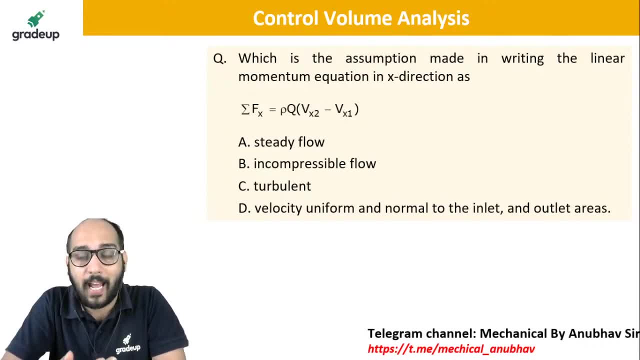 details. so if you have come up to understand, to learn something, to spend a little time to actually understand what this whole session is about, okay, hi arun kumar, very, very good evening. yes, i have. okay, so let- this is the first question, which is the assumption made in writing the linear. 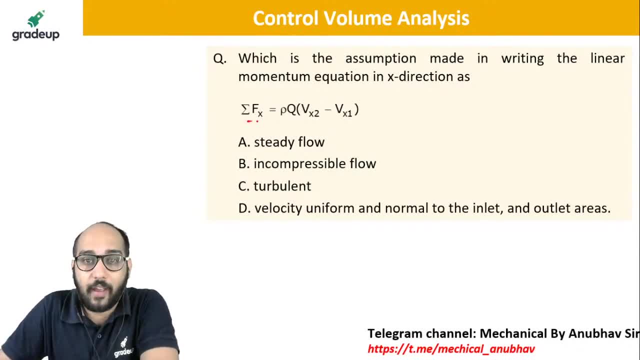 momentum equation in x direction. we know this, very famous. it's very useful not only here but when we move on to solve questions on hydraulic machines. the first chapter that we study is impact of jets- yes or no- very important as well as very famous equation. so what are the assumptions? 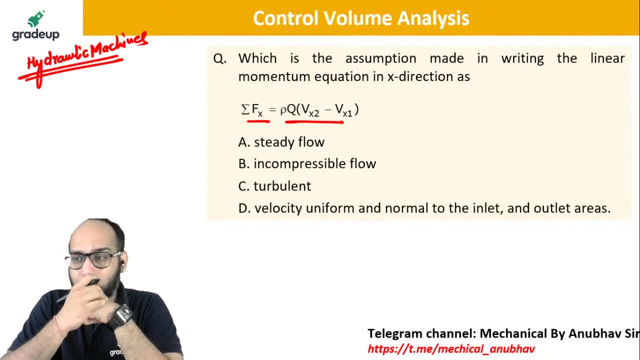 hi chandan paswan, very good evening, okay. so before you start, sir, let me help you out here. this is an msq question, okay so? so this is an msq question, so think wisely and then let me know what you think is the correct answer, which is the assumption made in writing: a linear momentum equation in x direction. 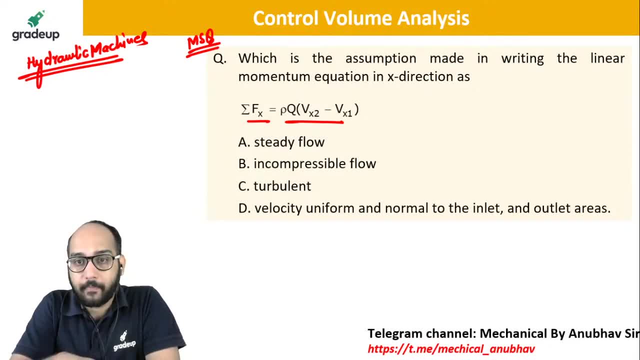 hi sandeep prajapati. hmm, confusion. try and attempt this question like this: which is the assumption? which is, which should not be the assumption? if i ask you which should not be the assumption made in writing, the linear momentum equation, then what would be your case? 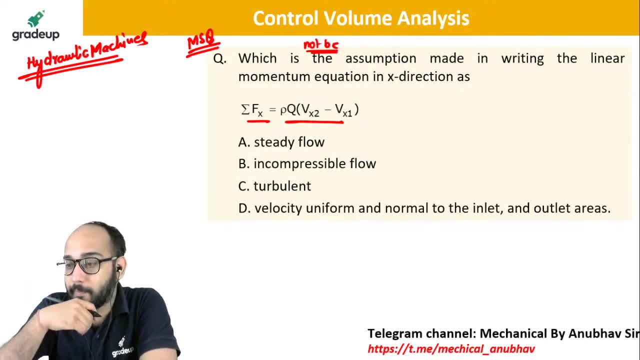 not, not the reverse of it, the negative of it. then it would be turbulent flow. okay, so this gets eliminated. it has to be steady, it has to be incompressible and velocity uniform and normal to the inlet and outlet areas. it does not say that pipe cannot be at. no, cannot be at angle. pipe can be at angle. 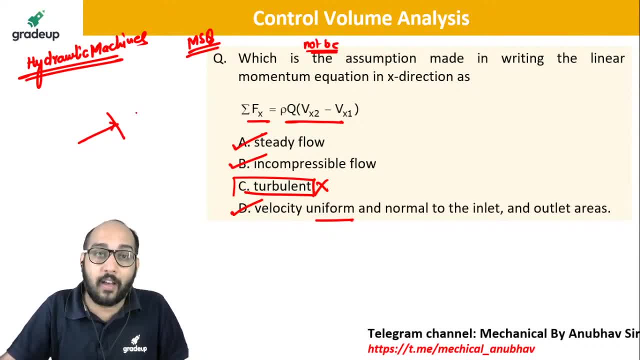 but whatever the outlet section is, velocity would be normal to it. this is what it's saying. whether you are discharging like this, so it would be normal. at an angle, it would be normal, understood. velocity, uniform velocity. sorry, it means they want to talk about uniform flow, kind of. 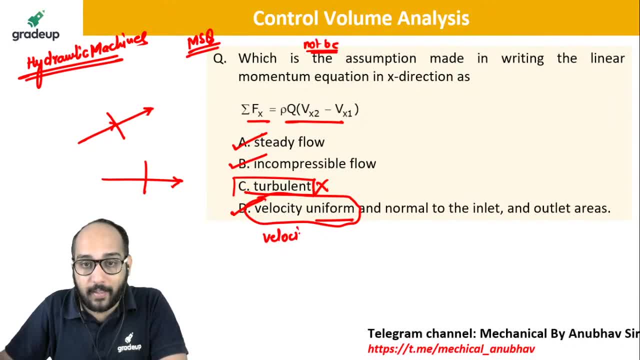 they. they are not seeing velocity uniform. only they are not. they are not saying that velocity should be equal, okay. they are not saying that velocity should be equal, okay. If you think so, then let me again try to rephrase this question next time. So may be you are feeling a little bit of vagueness. 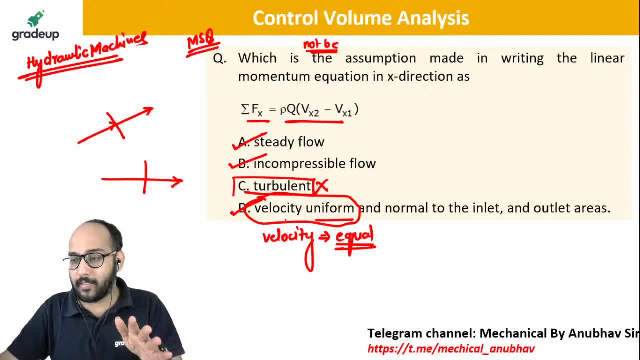 I thought this was kind of okayish. It's a little bit vague. Okay, I'll just rephrase it next time. Understood the concept, But you assume all the standard things that are still there to use this equation. Okay, let us now solve a question on this. 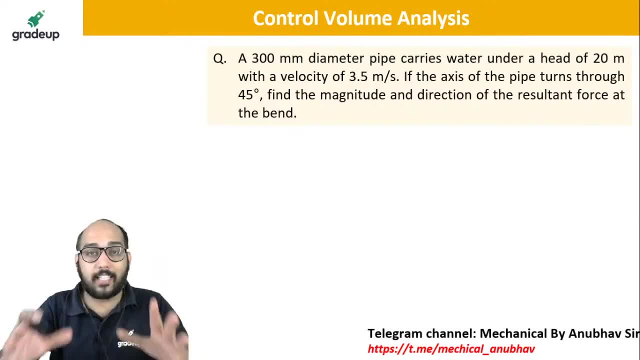 Okay, and we will try to. today I am directly jumping into the most important part. So our students say, sir, you always keep in loop at the end, the most important part. So today, first up, first good question is directly what we are there to understand. 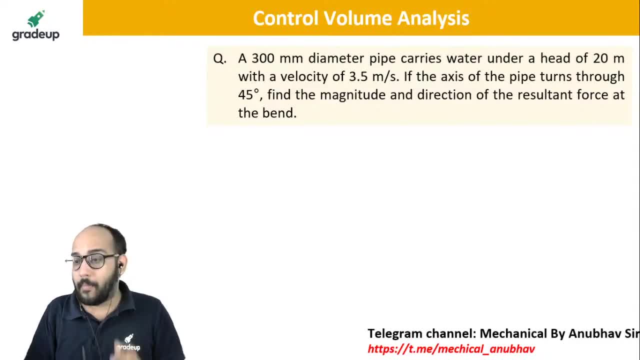 Not only this. We will have some good questions later on, But this is important. It says that a 300 mm diameter pipe carries water under head of 20 meter with a velocity of 3.5 meters per second. If the axis of the pipe turns through 45 degree, find the magnitude and the direction of the resulting force. 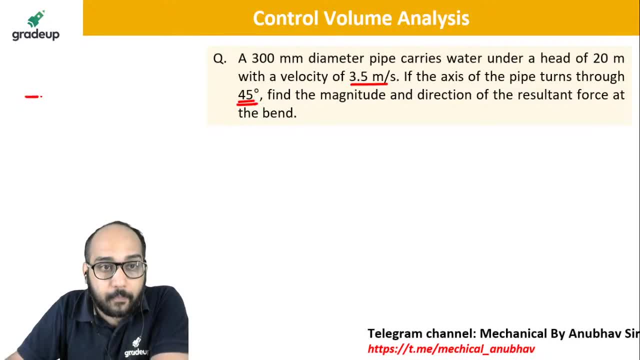 Okay. So if this is the pipe, Okay, This is the center line. This pipe turns 45 degree Like this: Okay, Sir, I can speak in Hindi, but the problem is that many students want to have this In English, and normally this platform may be discussing English, but I will just mix it up. 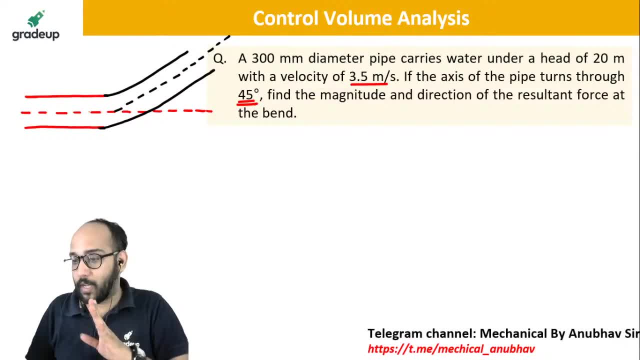 I will repeat it once in Hindi for you: Good, So this is the pipe that is coming, and then it takes a bend of 45 degrees- Again, a demand of only English. So we have this. I will just i'll talk about that later. okay, this angle is what? 45 degree. 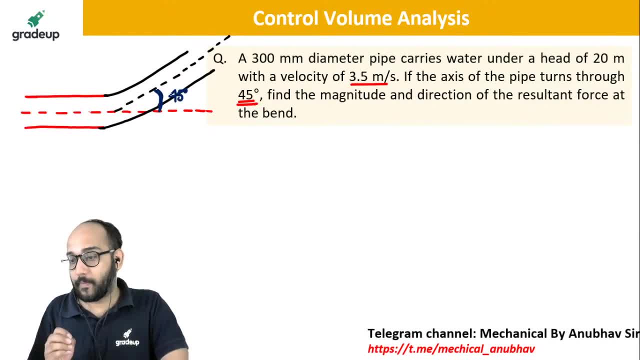 okay, never mind, we'll be doing it in english and you will never miss out any important part. don't worry, guys concentrate. yes, okay, this is the condition understood. so here the diameter is same: 300, same pipe, same diameter. so let us take section one here and section two here. 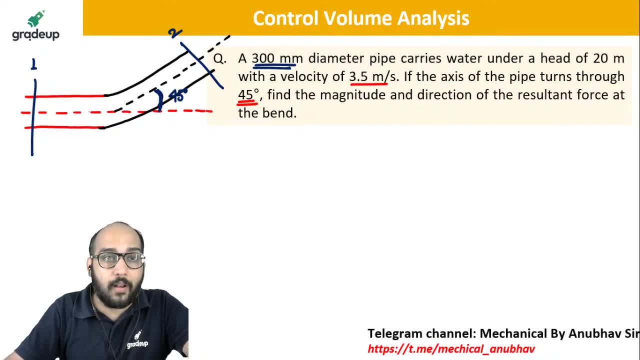 okay, so at section one, what is the diameter? d1 is equal to, d2 is equal to 0.3 meter. okay, the head is 20 meter, velocity is 3.5 meters. so can i see? can i see? the head is 20 meter, velocity is 3.5 meters, so can i see? 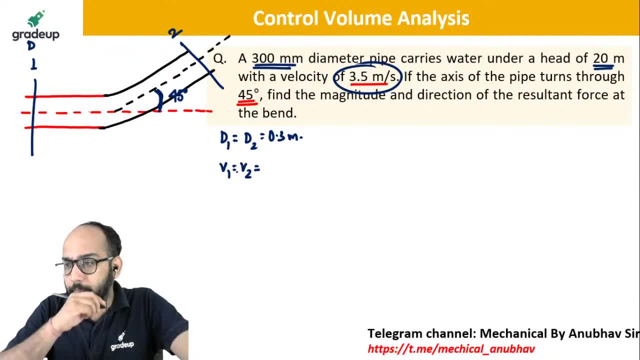 now directly say: guys, v1 is equal to v2. can i now directly say v1 is equal to v2? i'm smart enough now, sir, i've done continuity equation. okay, i will apply a1, v1 equal to a2, v2, since diameter is same. we are talking about water. it is an incompressible fluid density. 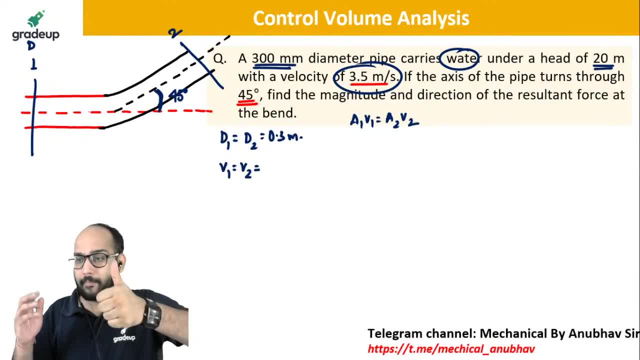 remains same: v1 is equal to v2. okay, yes or no? v1 is equal to v2, two linear. so let us start by assuming that we have an x one and up and v1 wealthy in the x one and up. if you observe, had the mentioned anything about elevation? had they mentioned anything about elevation? yeah, say, center line is 5 meter, 10 meter, 15 meter. have they mentioned anything like this? no, whenever they do not mention anything about elevation, we argue them to be at same height. okay, and generally, you will find the same thing. okay, so we will assume that the individualabso deze k. cordon to man aima hai. 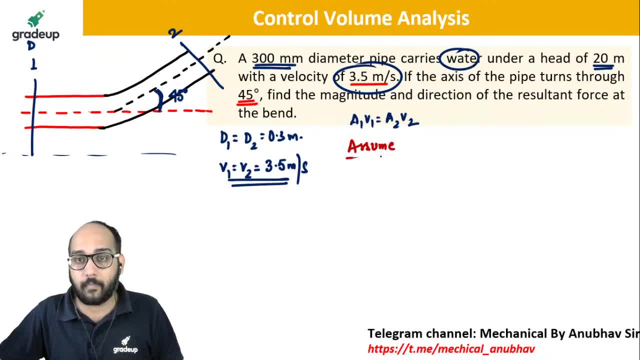 z1 is equal to z2.. Okay, Here also perfectly correct If z1 is equal to z2 and v1 is equal to v2. from Bernoulli's equation can I now directly say: p1 by rho g is equal to p2 by rho g. 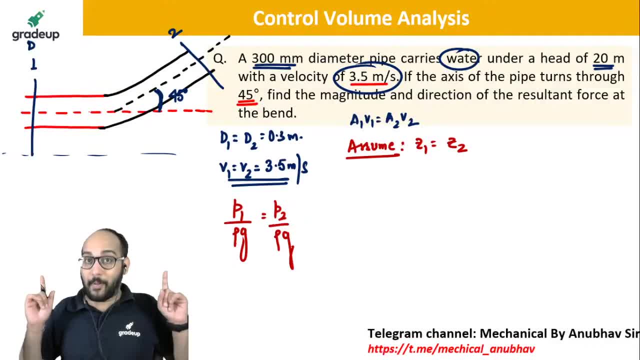 I am not applying it. I know I hope you are smart people, You know about Bernoulli's equation, But still Someone who has not attended. v2 by 2g plus z1 is equal to p2 by rho. g plus v2 square by 2g. 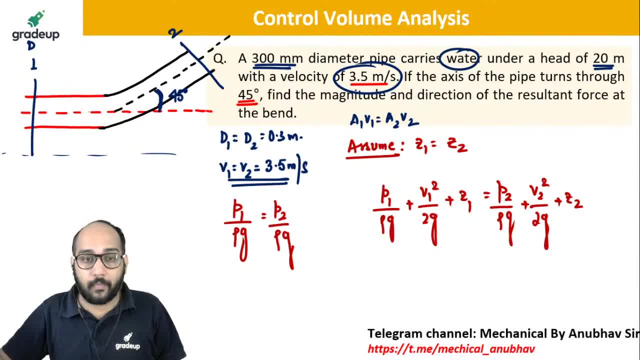 plus z2.. So z1, z2 we are assuming to be same. Cancel v1, v2. we again, we don't need to assume It is same, So this cancels. So p1 is equal to p2.. 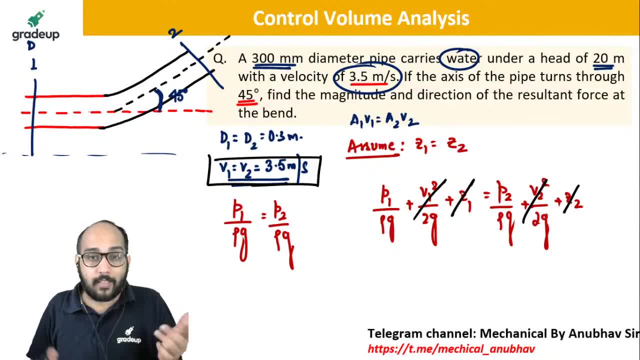 A very good question. UJ Styles is asking: Sir, what about 20 meter head? What is fair, This is your 20 meter head. So from here, what do you get? This is nothing but 20 meter of head. What is p1?? 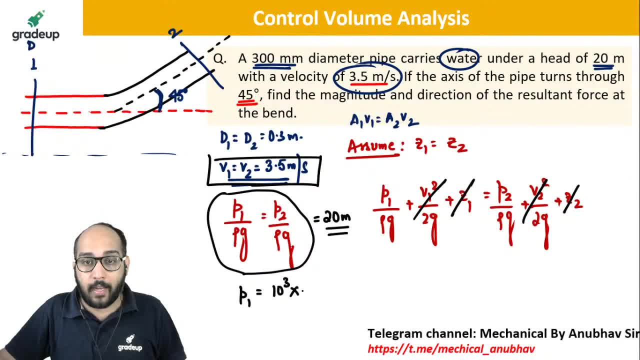 p1 is density 10 to the power, 3 into 9.81, into 20.. How much is this? 196.2 kilo Pascal hobby, Get it. So what is this 20 meter of name? This helps us to calculate what is the pressure. 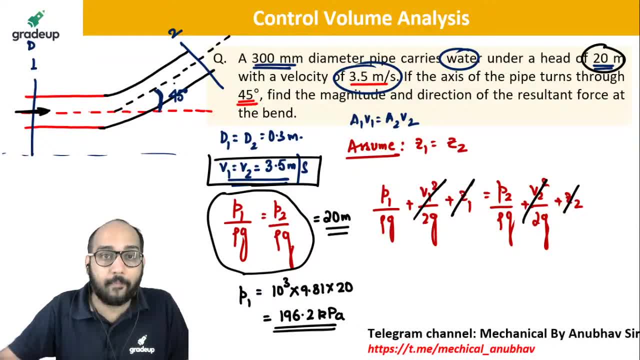 So with this pressure, fluid is entering and this is p2. So we have concerned recombination. So the values are perfectly clear. Yeah, I have mentioned in kilopascal. The values are perfectly clear. Now let us analyze this. So the idea is very simple. We will apply. 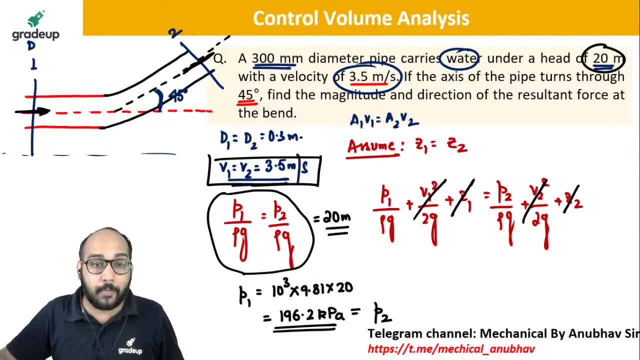 impulse momentum principle. What is impulse momentum principle? It is: summation of fx is equal to rho into q, v2x. v2 means, at the exit velocity in x direction minus inlet velocity in x direction. Okay, Now, before we start to apply this, what are the forces that are? 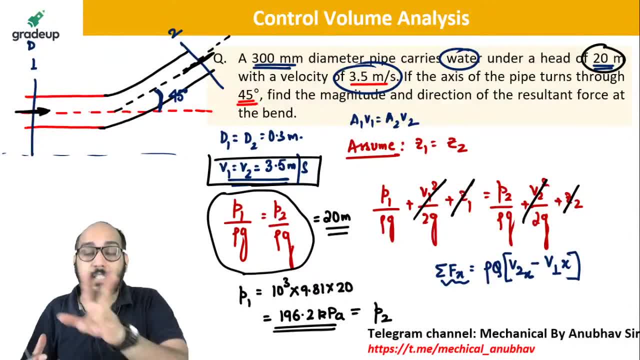 acting, or what are the directions of forces and the velocity. So, before we start, what do we assume? We assume that This is the force fx, which is applied by what? This direction fx and fy. Now tell me guys, what is this force, Fx and fy? Sigma means summation of forces in x direction, Sigma. 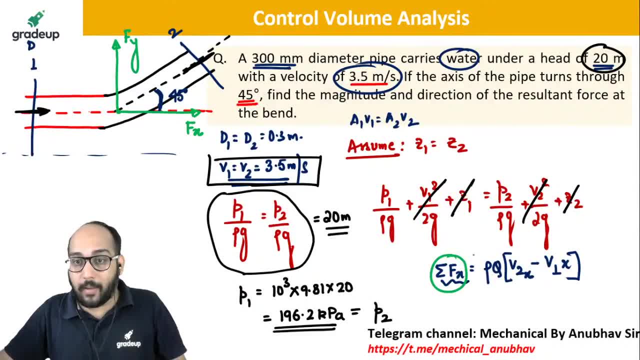 of forces in x direction. Okay, Summation of forces in x direction. Okay, So this is fx. Okay, What is this fx that we normally take? Okay, So these direction we normally assume this is the forces that is applied by the pipe on the fluid, No, by the pipe. 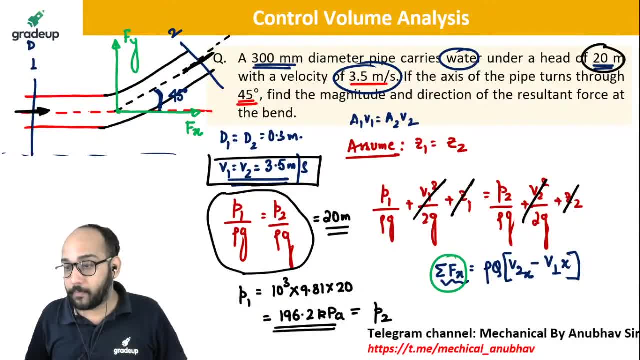 on the fluid. This is what we assume. This is impulse momentum principle. Okay, So, this is my finalement method, which already is been used in the last video. Okay So, with the Torah example, friends, let me give you the. 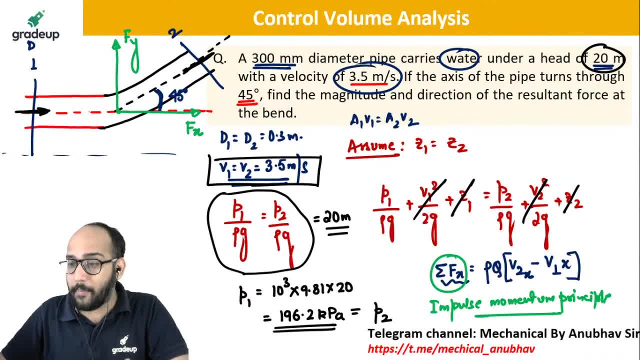 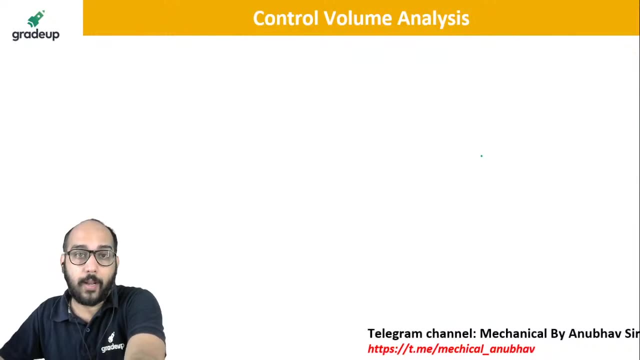 first 불ion right In another verse. Okay, it is coming from a little bit of your second law of motion. okay, we apply per unit time. we get this relation. okay, now let us talk about it. so if we talk here, I'll just draw the pipe flow again and please understand. first question: 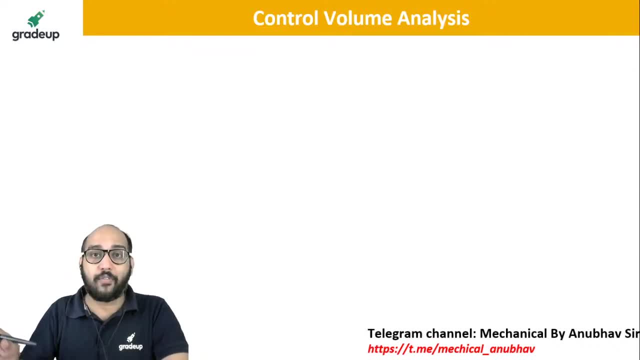 we are taking some time so that we understand it once and for all. after that we don't want any problem. so this is the inlet. this is my section bar. when the fluid is entering, pressure force acts normally, yes or no. pressure force acts normally. so this would be the direction of P 1. 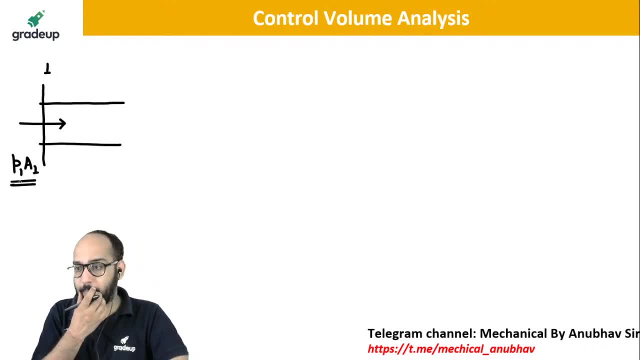 into a1. pressure force acts normally at the inlet, okay, and it is entering, even it will when it is leaving sat an angle. what is the angle given? 45 degree, okay, so we are talking on the fluid at this time. the yeah page of who we took a sad 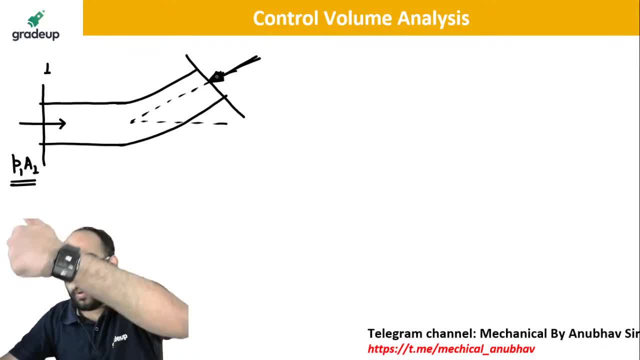 path, So P2A2, so its reaction would be in this direction. P2A2, yes or no? For me this is the control volume, This is my control volume. Anything outside I don't care. This would be P2A2 in this direction. 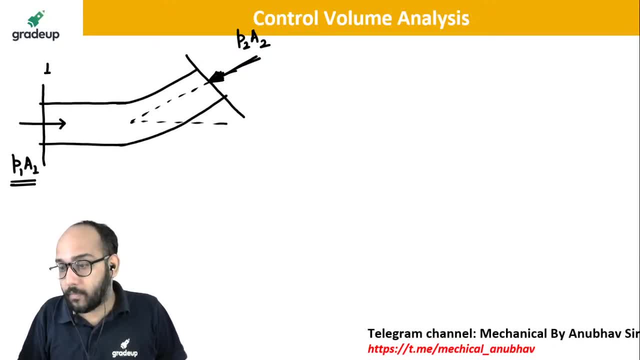 Sir, how many V1 and V2? V1 equal to V2, that will be cancelled. Now, what is the angle This? This is the same angle this. See, if this is theta, This would be theta ok. 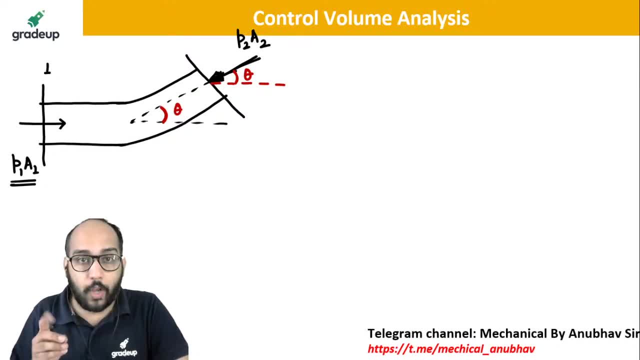 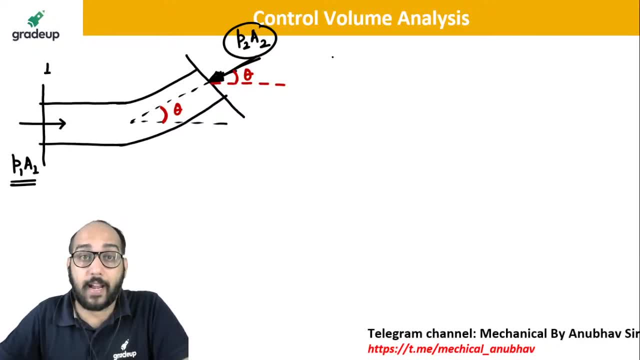 Ok, so this is P2A2 in this direction, P1A1.. So if I die and another one that I am taking is Fx in this direction, Ok, and Fy force in this direction. So what is the net summation of forces in x direction? 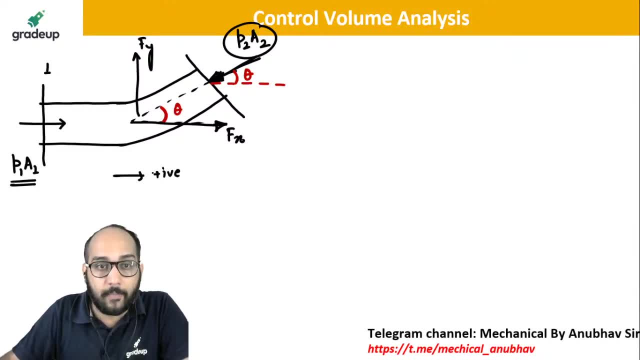 So if I take this direction as positive, Yes, Yes, this direction is positive. so how do i write it? fx right first. so this is p1 a1 plus- this is in right hand side- fx minus p2 a2. but you want in x direction. 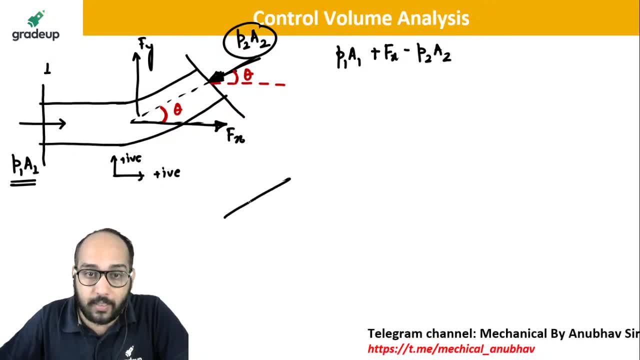 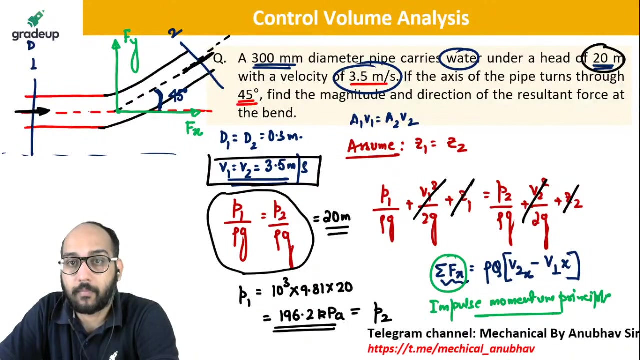 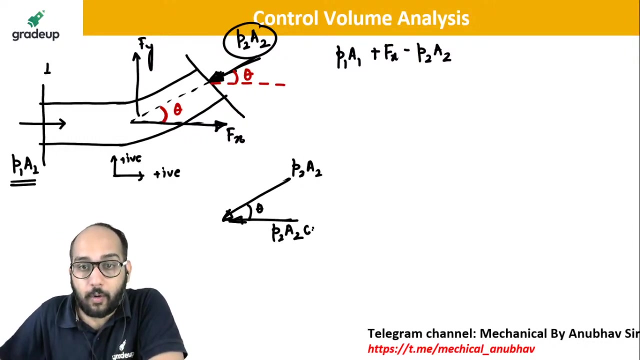 horizontal. if you take the component of this p2 a2, is this: this is angle theta. what would be this? what will happen? p2 a2 cos theta or sine theta? this would be p2 a2 cos theta, sine theta. ok, so this is p2 a2 cos theta i. this direction is this side, left hand side. 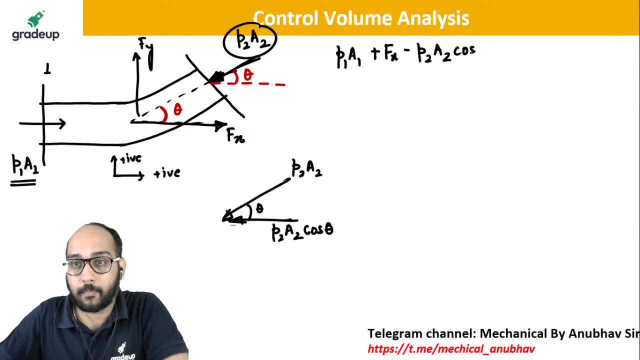 going left hand side. so this would be minus. this is equal to row into Q. now, final velocity in X direction. now, if you draw the direction of velocities, this is that the direction of velocity at the exit. this is the direction of velocity at the exit, v2. 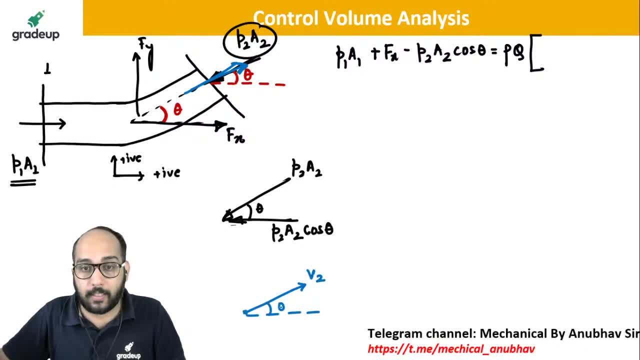 with the horizontal. this is theta. so this would be what v2 cos theta in x direction agreed minus at the inlet velocity is in this direction only. this would be v1. understood how to formulate the equation. we will also take up one case. you would say: sir. 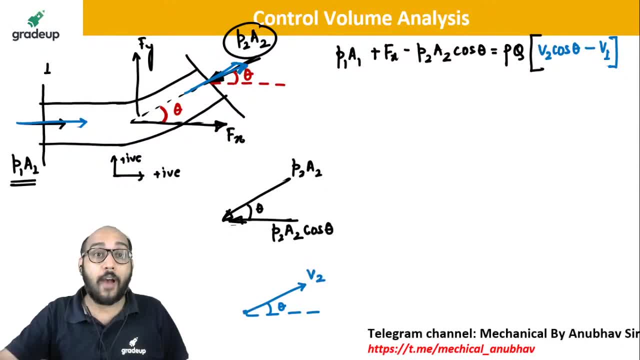 this is very standard. we know what if you have an angle of 135 degree, say this is the next question. okay, so i will complete everything, don't worry. okay, so let us now put these values. we all know what are the values, so very quickly put this value and calculate the value of fx. 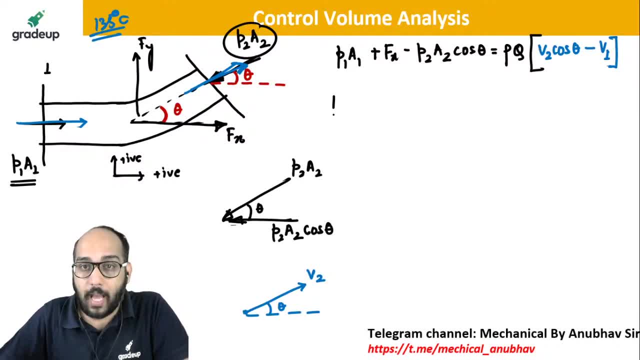 so from here i can take p1, a1 to be common. i get 1 minus cos. theta plus of fx is equal to discharges area into velocity: v2 cos theta minus v1. now we know v1 we 2 is seen the. can i not take this outside? 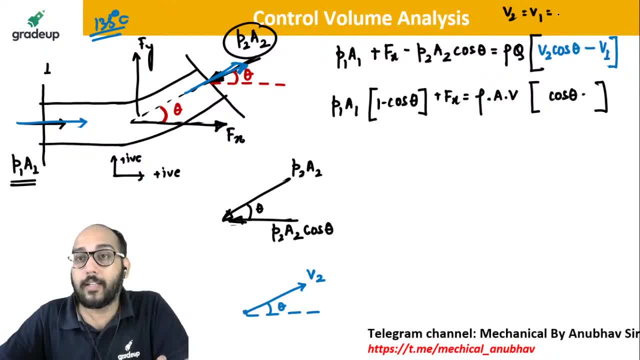 we know now, v2 is equal to v1 is equal to this muchv. this will be v squared cos theta minus 1.. ok, so you know these values very quickly. limitations can be done very quickly. no, tell me what is the value of fx. 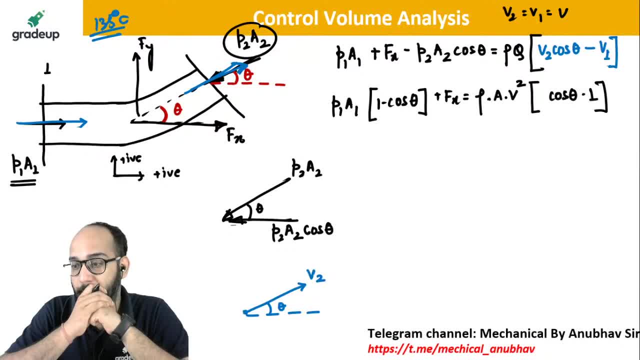 there is one thing i would like to ask: how many of you do think, sir, even and this a and this a can be cancelled? yeah, we always take gauge pressures. we always take pressures. we do not take, take into consideration the atmospheric pressure. there is another one, numerical, like nozzle type, that has come in gate. 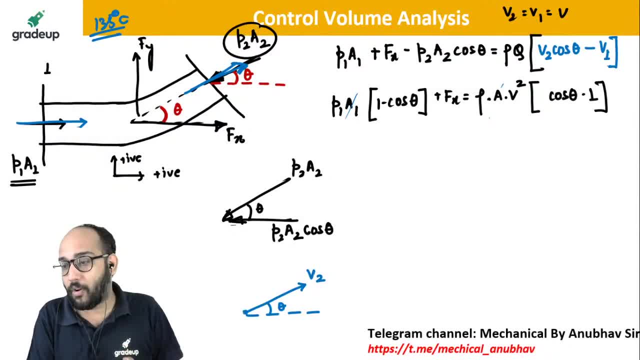 exam. so again the same principle we have already discussed. to take gauge pressure, how many of you do think he said this area and this area can be cancelled? don't get, don't be afraid of those who think you are saying no, have like in the first few. what happens is when we try to do quickly, we see a, a, both. 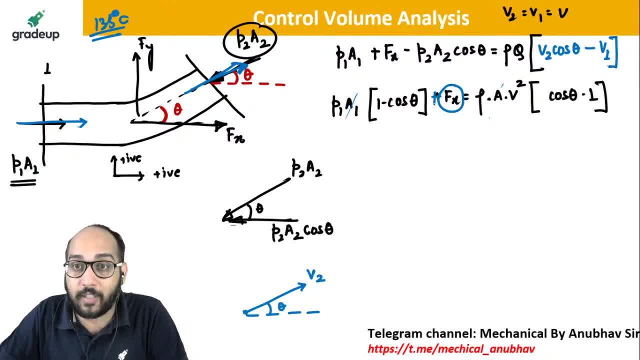 sides. we cancel, but we forget that this term is with plus. it does not have a area, so you cannot cancel it out. if you are cancelling, you have to divide by area, okay, so this is a common mistake when you are trying to solve these kind of questions. 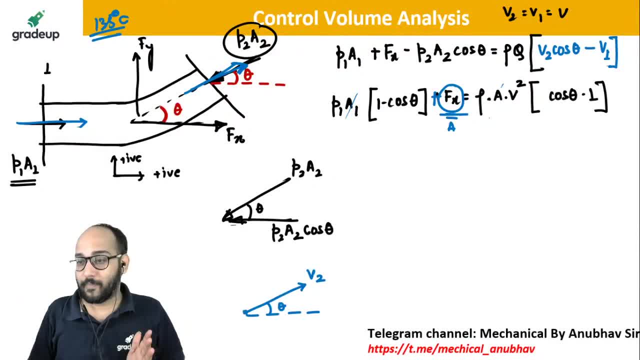 quickly in the exam. you make these error, okay, so don't do it. you might, you, i might sound to be very putdu, sir, yeh sab toh, i know hai who makes these mistakes. believe me, people do make these mistakes, see, if you remember, just remember the formula. 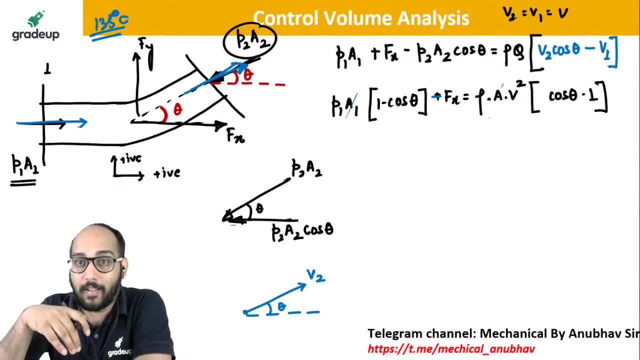 everytime. it is not applicable. if you formulate fx from here the next question, there will be changes in final okay. so i am not telling you to remember the formula. remember the basic impulse momentum principle, net instructors in x-directions or white direction is equal to 20 into changeable. remember this anymore, devailleurs. 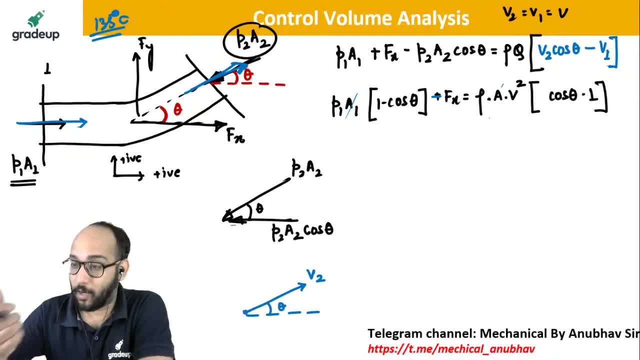 yeah, See, I made a mistake, isn't it? That is awesome that you are honest. It happens, guys believe me. So let us put the values 196 kilopascal, So 196.2, into 10, to the power 3 into area. 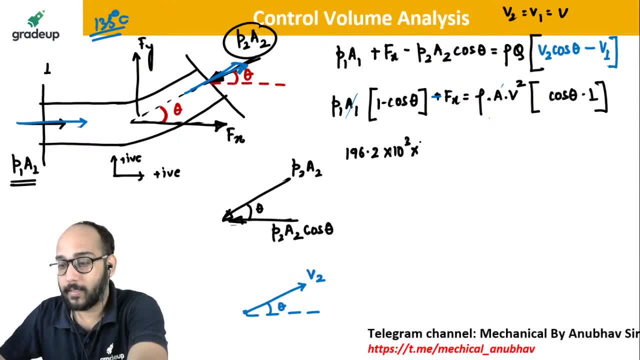 Area is pi by 4 d square, or something like this. That is the principle. Absolutely, Sandeep. Thank you, Come on, come on, guys. What is the value? It seems like a very lengthy calculation, Do you feel this? 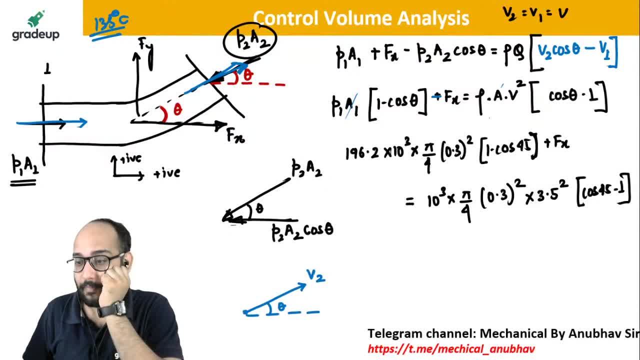 That, sir, this is a very lengthy calculation To solve. to reduce this: now understand how are we doing So? I do not want to multiply this very complicated thing twice. I do not want to multiply this very complicated thing twice. So what do I do? 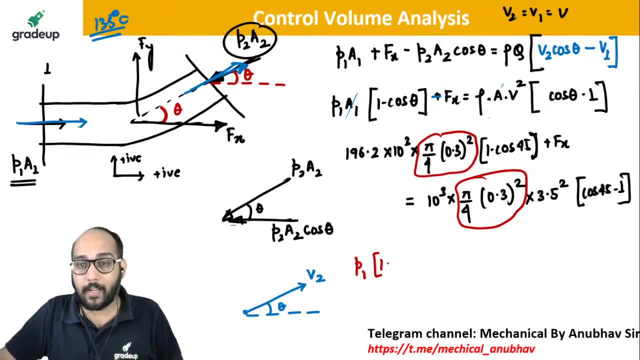 I take p1, 1 minus cos theta, which is comparatively easy to calculate. Write it fx by: a is equal to rho into v square cos theta, Theta minus 1.. Okay, Now understand. this is in kilopascal, This is a kiloterm. 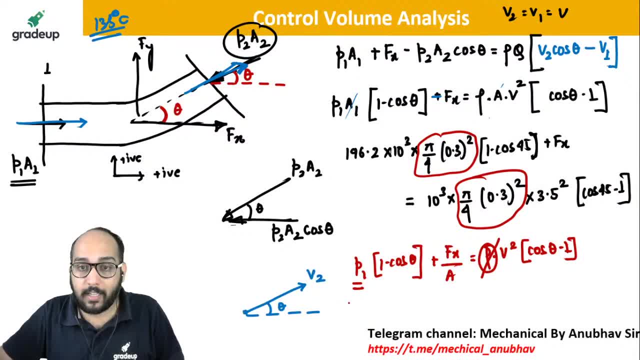 So if I cancel rho and just write 196.2, 1 minus cos 45. I am by default calculating this force in kilopascal. I am by default calculating this force in kilopascal. Understood: See here: 10 to the power 3 term comes. 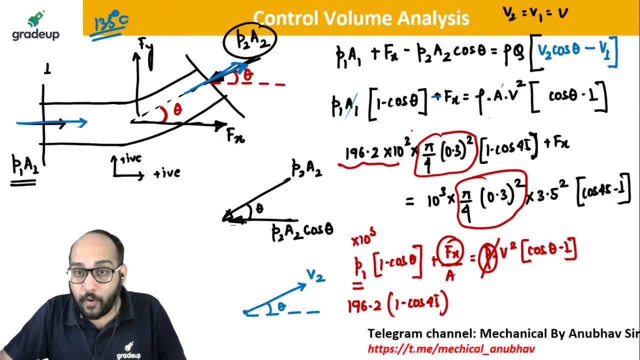 If you split, as I have written here, If you cancel 10 to the power 3 here, 10 to the power 3 here, You have to divide fx by 10 to the power 3.. Which means fx? answer would be in kilopascal. 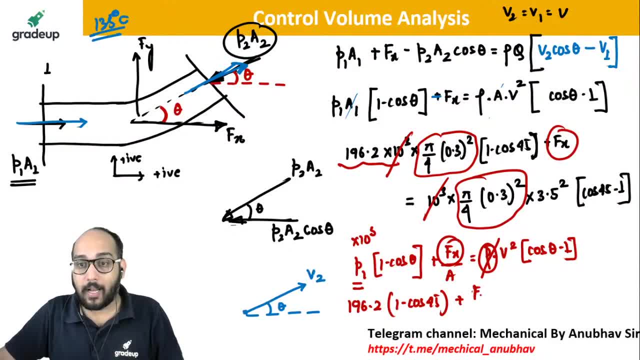 Okay, So plus fx upon of a is equal to 3.5 square cos theta minus 1.. Now it is still easy to calculate. So first you calculate this: This subtract karo multiply by 5, by 4 d square. 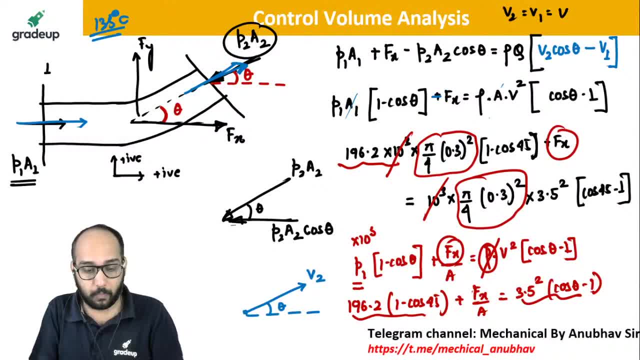 How much is it coming, guys? Yes, fx is coming as minus 4.2.. minus 4.2., That is 4.31 kilonewton, And this is my dear friends gate. exam question is straightforward. You still know the formula. 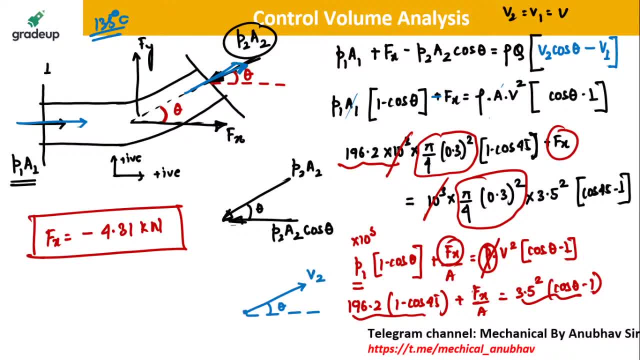 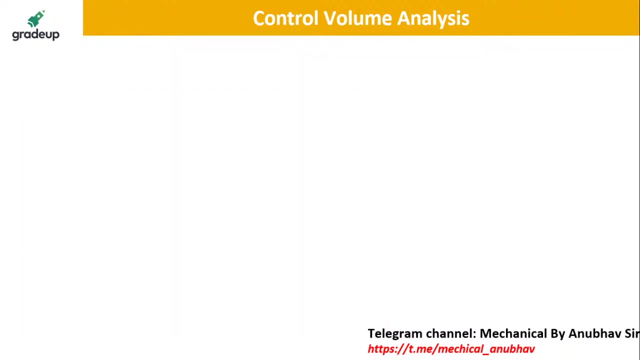 Look at the intensity of calculation. Okay, So fx is 4.31 kilonewton. Good Good, So fx is 4.31 kilonewton. Okay, okay, yes, absolutely so. this is fx. now. similarly, if we try and calculate for fy, 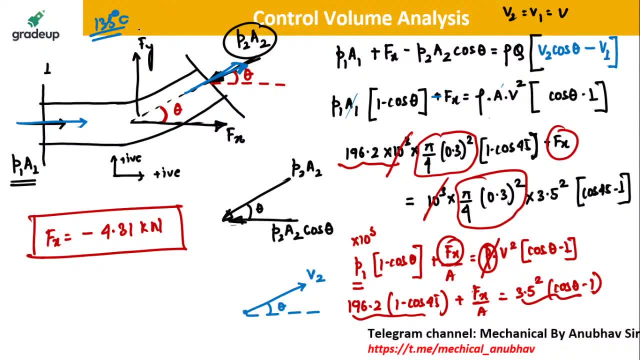 f? i equation. here let's write direction of forces in fy. now in x direction. there is no force in y in, sorry, at inlet one, there is no force in y direction. so this would be zero. okay, plus we are taking this direction: fy positive plus of fy. 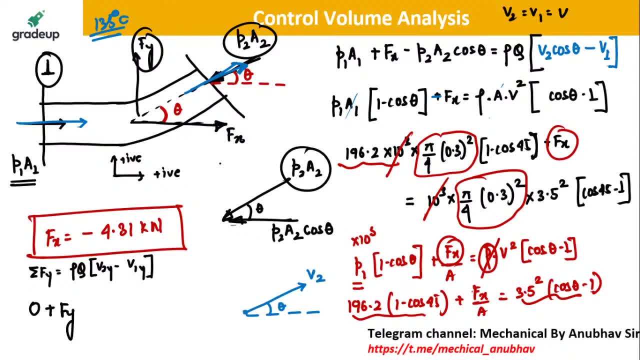 now, what is the direction of p2a2? in vertical this would be p2a2 sine theta minus p2a2 sine theta is equal to rho into q, v2 in y direction. so v2 in y direction is this. how much is it? v2 sine theta. 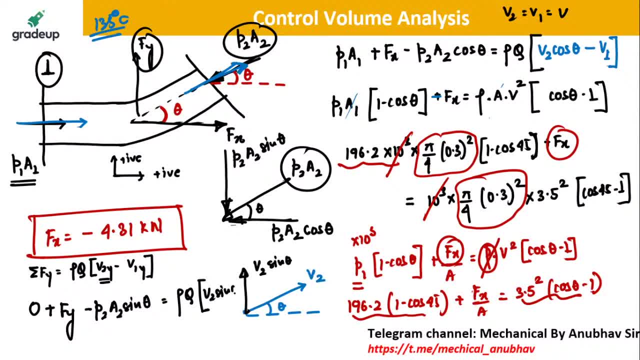 v2 in y direction is this: this would be v2 sine theta, minus at the inlet velocity in y direction. that is zero. this is v2 sine theta. so from here what do you write? fy is p2a2 plus rho, q, v into sine theta. 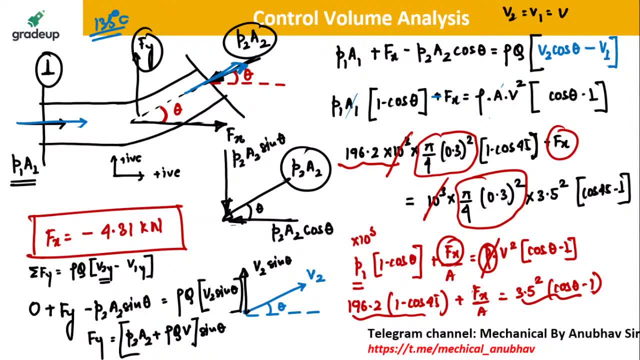 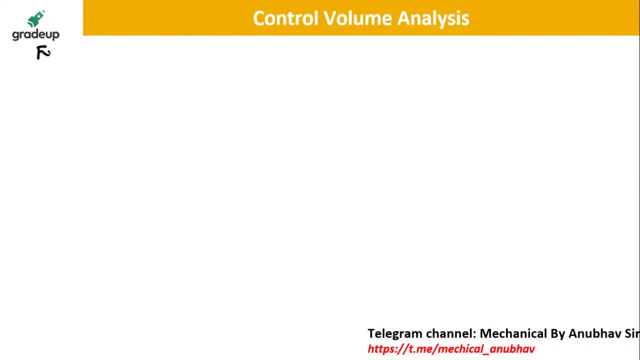 okay, calculate this value, guys, come on. fy is p2a2 plus rho into area, into velocity, square, square sine of theta, sine of theta f y, f, y, f, y, guys, come on, is 10.4. no, we need just do calculation, making some mistake: 10.418. 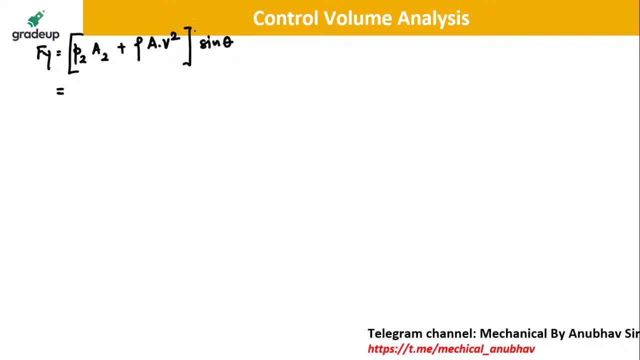 if you take the area common, you get 196.2 plus 3.5 square and then you get 10.4 area pi by 4 b square into sign 45. whatever you get, the answer would be in kilopascal, didn't I give you some priests. 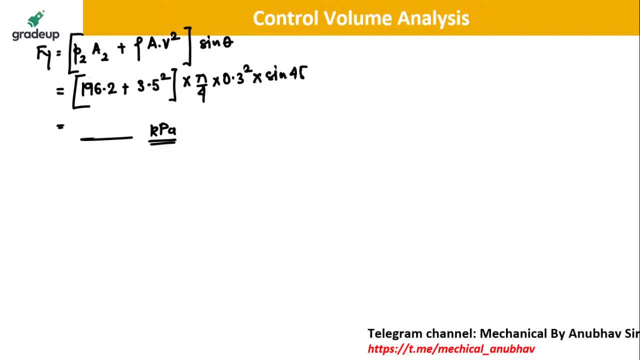 but you're a god knows who's involved in. you need to give me a thing like this, because if, when I go back in time days, I'm going to say a bunny snap, squat, your heart would go crazy. then there are other stories about me knowing that. 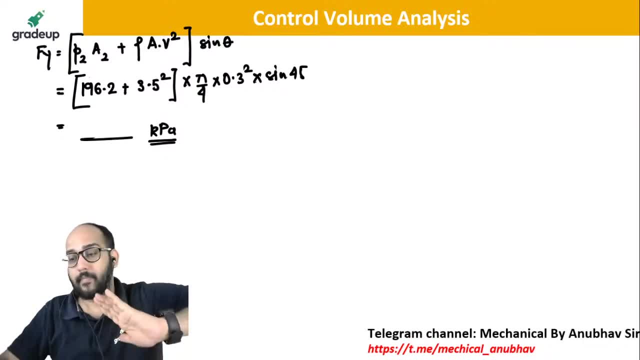 yes, I'm never Kendra. the theory behind a zebraед is just a myth. all right, buddy guys, as ten point four, one eight, do we all agree? what do you say you should do? it? option is: yes, it is ten point four, one kilopascal. 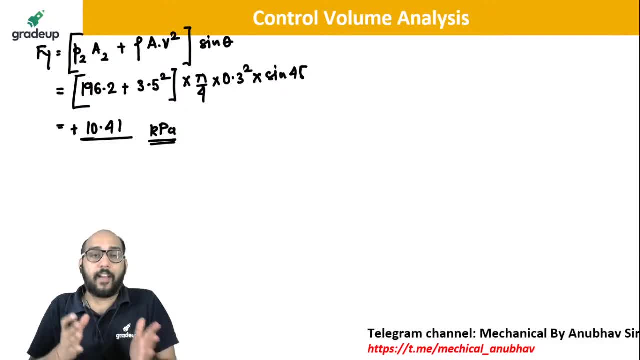 okay. so once you calculate fx, you want to calculate fy. what is the resulting force? is fx square plus fy square? you calculate resulting. what is the angle? tan theta is fy upon of effect. we calculate the angle understood water. water is given. water is given. rho is thousand. 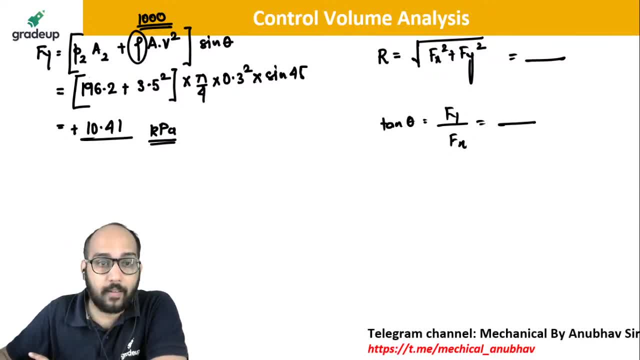 okay, so i'll write it up here into ten to the power three and row ten to the power three i've taken out and then convert it into kilo. okay, rajesh babu understood. so what is this value coming as? finally, eleven point two, seven kilo newton, and this angle is coming around sixty seven point five degree. 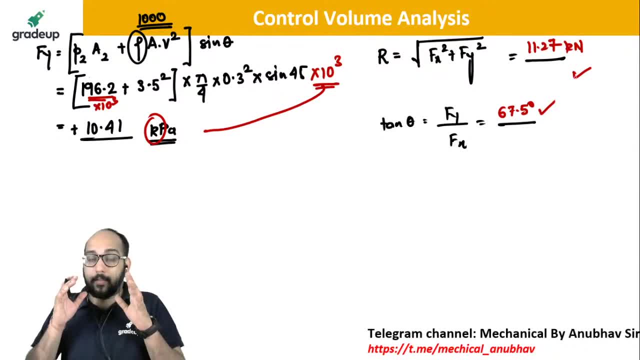 so this is how we go on to calculate. so this is how we go on to calculate our impulse momentum or a pipe bent equation problem: exhaustive, lengthy and please make sure that you do not make a mistake- two marks question. may, sometimes it do appear, but, sir, do we remember the formula? always remember what was the formula that it was coming. 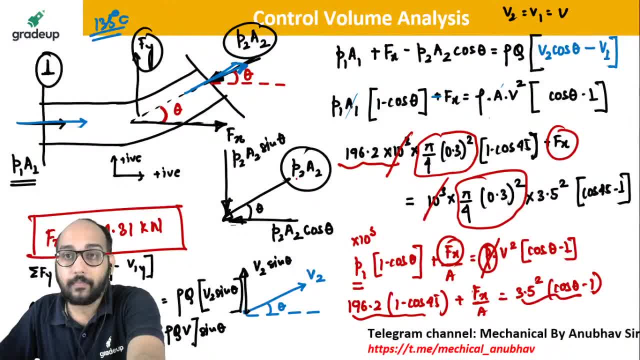 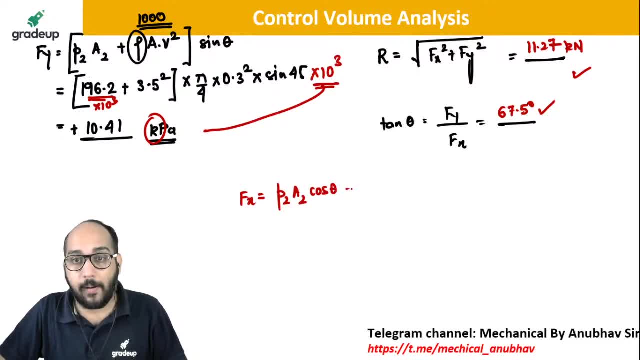 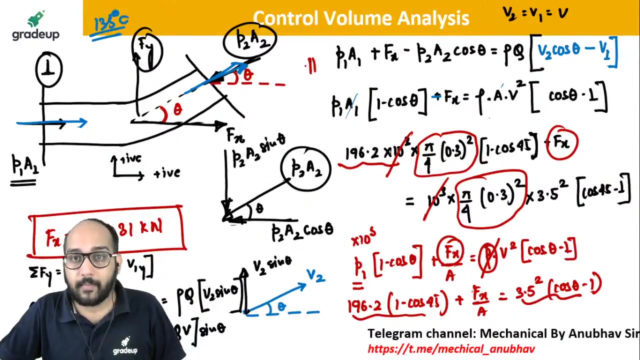 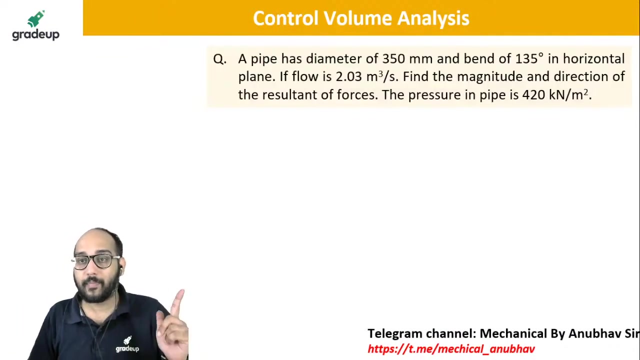 fx is equal to, if i write it down: v2- a2 cos of theta minus p1, a1 plus rho q. v2 cos theta minus v1. this was the formula. if you just remember this formula and try to apply it in this question, okay, the question is exactly the same. is of 350 mm, bent of 135 degree. this is exactly the same, so that was the right formula for to get that up. start with this one. longer, a type has a diameter of 350 mm, bent of 135 degree fence, and it's also a 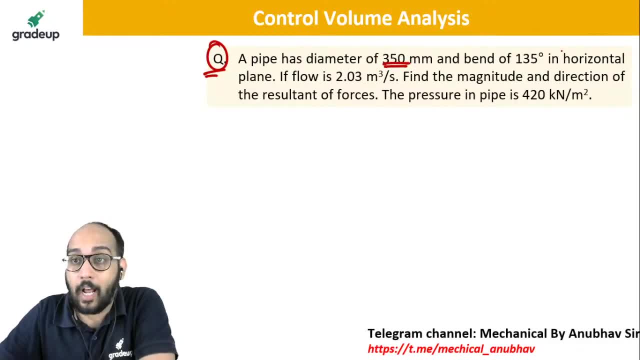 type of hydrolyzed area of 350 mm is. it's builded on the pipe. this is the type of beimuseh resistance in this mine is bovava. is there a violation? the afraid amigo was teaching aTimberjackược. in horizontal plane flow is 2.03 meter cube per second magnitude and direction of the. 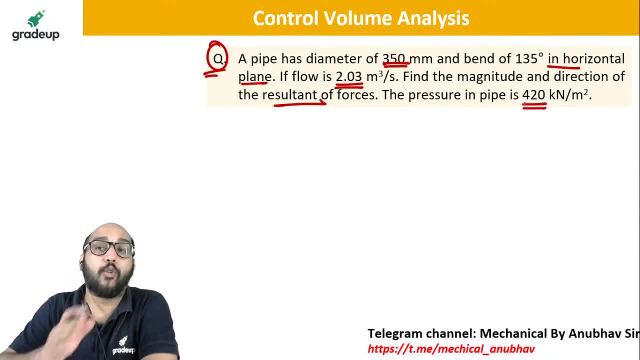 resultant of forces, if the pressure is 420 kilo Newton per meter square. So what does it say? that you have a pipe, constant diameter and there is a bent of 135 degree, a bent like this, something like this: if you measure this angle, this angle is 135 degree. understood the diagram diagram clear. 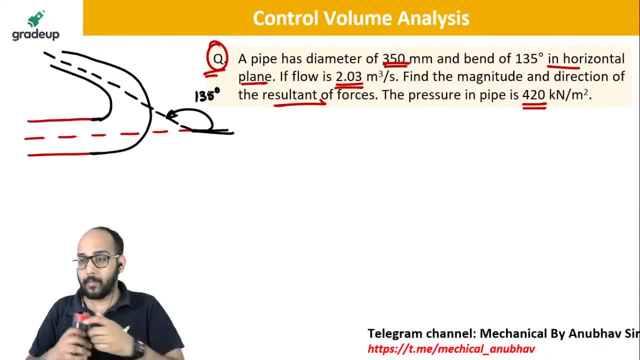 It is like the road that you go on for a mountain: go to Uttarakhand, Himachal Pradesh. you can find like these roads, ok. So is this diagram clear? Now let us see If you see, diameter is same. D1 is equal to D2, 0.35 meter. so can I say A1 is equal to 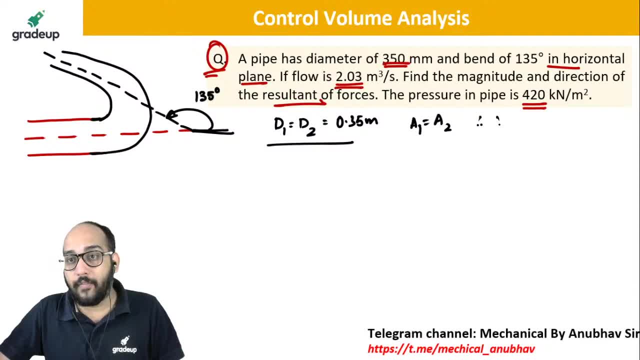 A1 is equal to A2, so therefore, B1 would be equal to B2. ok, What is this value? you can always calculate 4 cube by pi G square. you know how to calculate it. ok, B1 is equal to B2. applying Bernoulli's, you get B1 is equal to P2.. 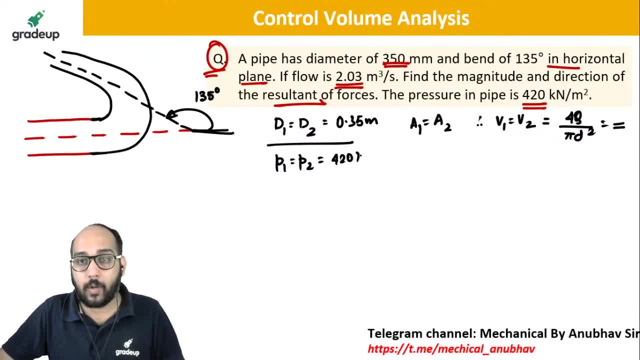 Which is 420 kilo Newton per meter square. This analysis we have already done. Now, what is so special about this? The special thing is: how do you formulate the equation? What is the equation? It is: a net forces in x direction is equal to rho cube velocity at the exit in x direction. 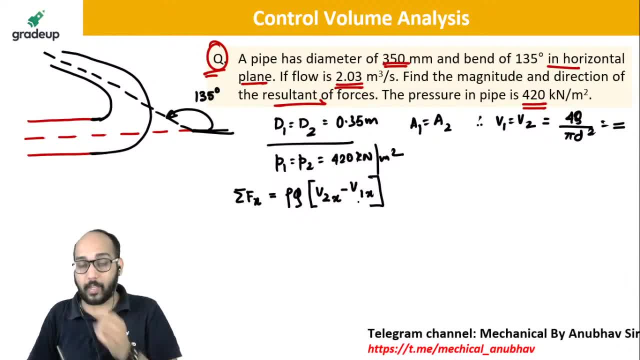 minus velocity at the inlet in x direction. Ok, Let us try and formulate this. ok, If you formulate the equation, then you know how to solve it. time lagega, but ho jayega. So this is the section 1. this is the section 2. ok, 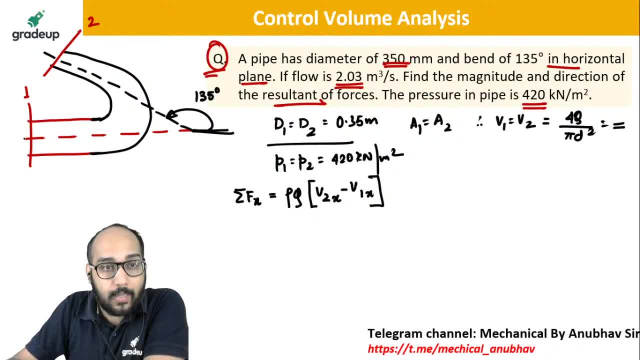 So if I talk about section 1, this is pressure force P1 A1. agreed, This is the section 2.. Ok, Ok, So this is pressure force P1 A1.. This is Fx forces on the fluid by depend and this is Fy ok. 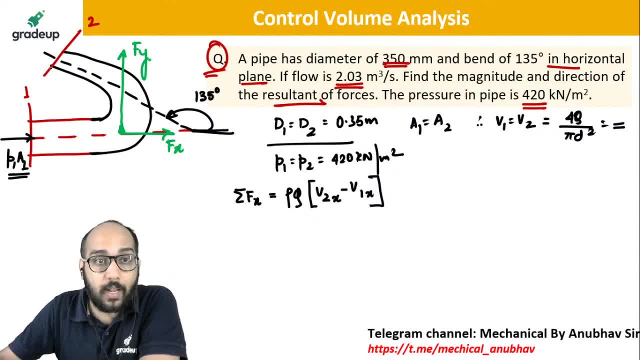 And what about P2 A2? now look here: the flow is in this direction. the flow is in this direction. So the action P2 A2 will be in which direction? this direction? P2 A2 would be acting in this direction, yes or no? 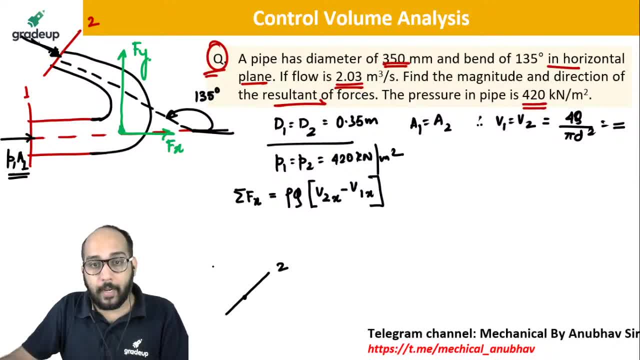 This is the exit point 2.. Then P2 A2 is acting like this: Ok, Ok, 1,, 2, 5, 4, 7, 8. which direction is this Now? this is the exit point 2.. So this is P1 A1 x, P2 A2.. 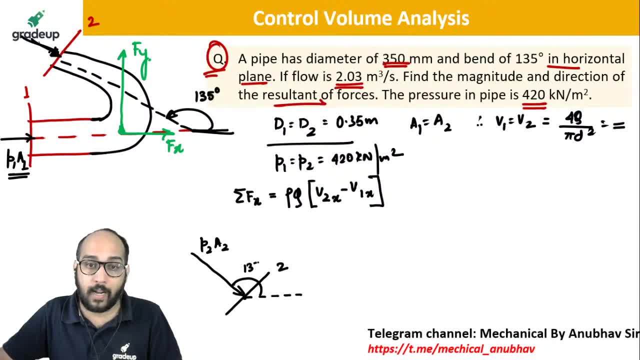 Now, what is the angle with the horizontal angle? is this 135 degree? This is how much. This is how much saw. Now, this is this is how much: 45 degree. now you try to put the equation p1- a1. we take this. 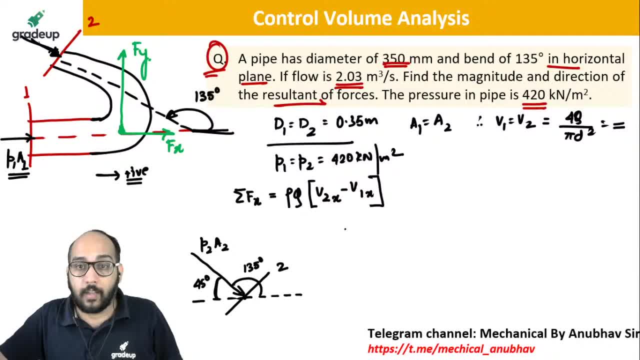 direction as positive. so p1- a1 is positive, plus FX. now what would be the sign of p2- a2 which we are to take in X direction? so in X direction, this would be p2, a2, cos theta. what is the direction? this is the direction, sir, right and side. 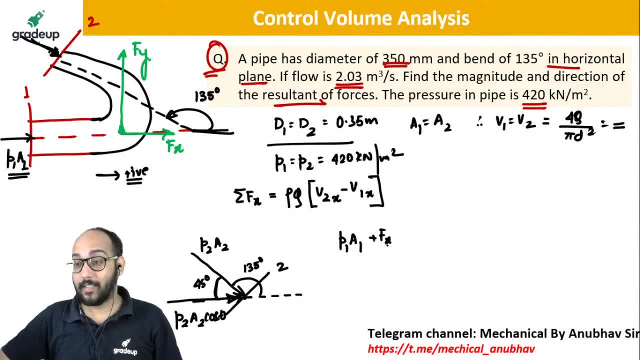 we are a plus or minus. plus, okay, awesome, I haven't done the calculation. so whatever you guys says, you say, I will agree with the answer. so this is rho Q velocity in X direction. now flow is in this direction. this is the direction of v2. what would be the direction of v2 in? 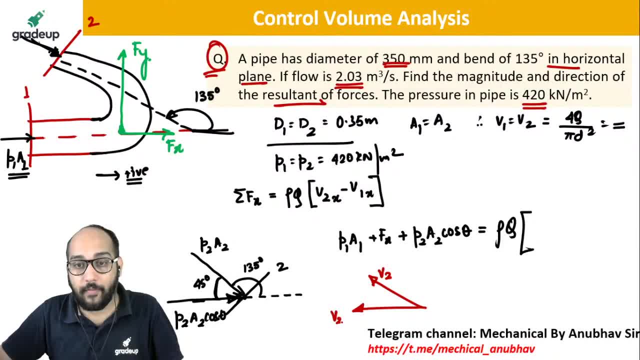 X, this. this would be v2 X, which is v2 cos theta. this will be minus v2 cos theta. okay, minus v2 cos theta, minus of, and the course is always taken. this is basic. what do I say? vector or basic thing? now, Rajesh, you are taking the base on which side? if this is the hypotenuse, 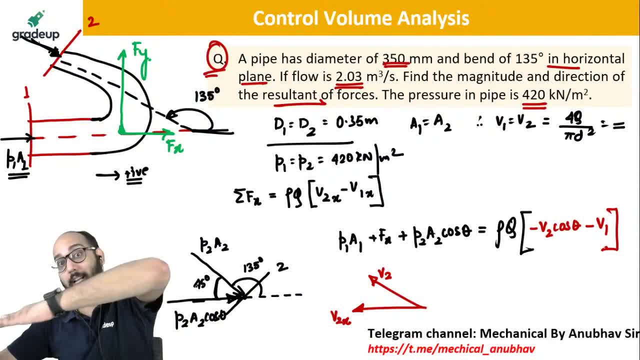 this is the base that you are taking now. you're not going this side. this is, this is what you are taking, the component. so yeh kis angle pe base banayega. yeh aise ghoom ke idha thodi na jayega. this will not go in this direction. this is p2a2, if it has. 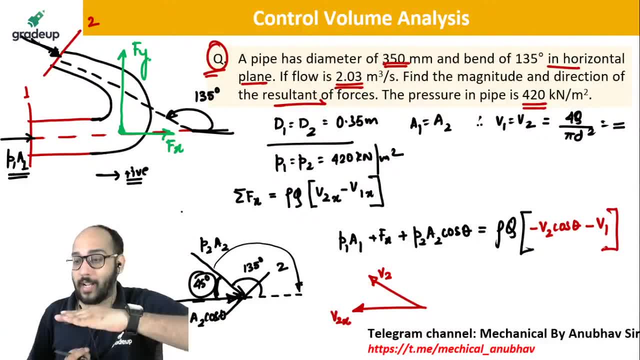 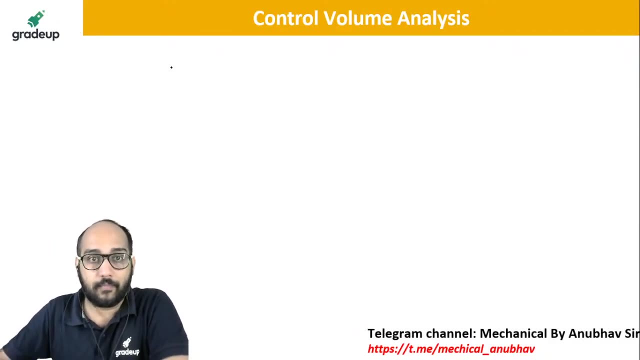 to: you want to take the horizontal component, you will take this component, understood. so this is how you formulate this equation. rest is easy to solve. okay, let us talk about f y, f y. so this is the direction of p2a2. okay, two point. so component here would be what? 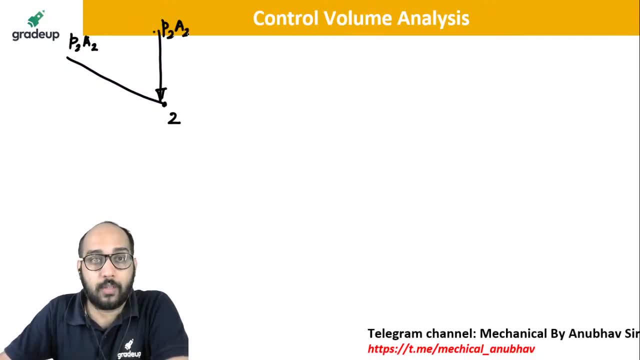 p2a2 sin theta. what is theta? this is theta. so if you try to calculate in y direction, we write f y. f y is taken as positive. this would be negative. minus p2a2 sin of theta is equal to rho q, now v2 in y direction. 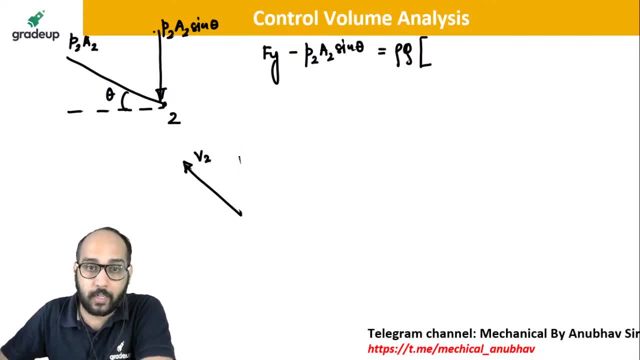 this is the direction of v2, this rho q. this is the direction of v2, this rho q. this is the y direction. this would be v2 sin theta. so this is going upwards positive inlet where the y direction is zero hai. so this is your equation to calculate f y. understood so this? 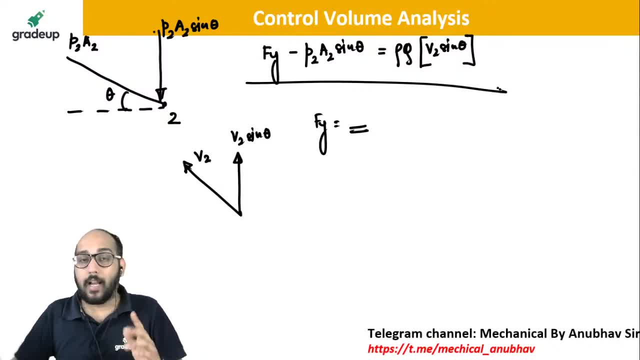 is very, very important. you do your calculation guys and take this sine theta. so this is the you do your calculation guys, and if any doubt, this is the telegram channel. okay, you can post your doubts here. I'll be happy to help you out, okay, so try and. 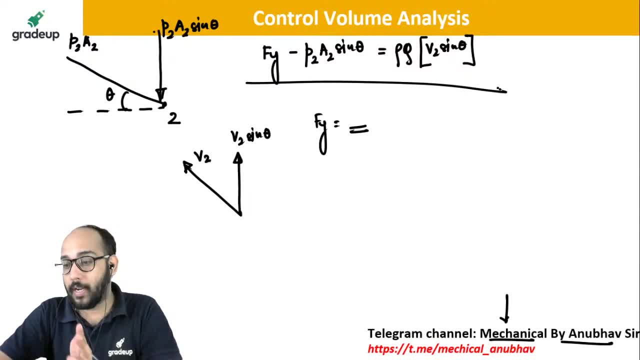 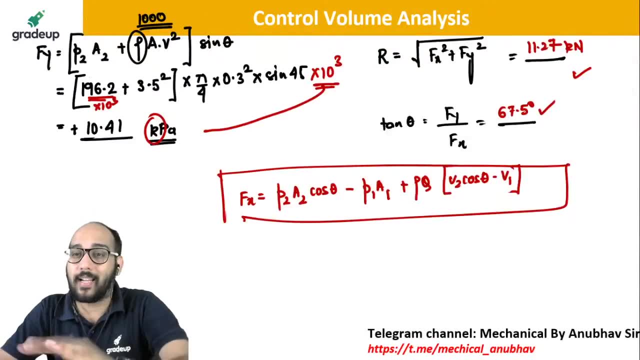 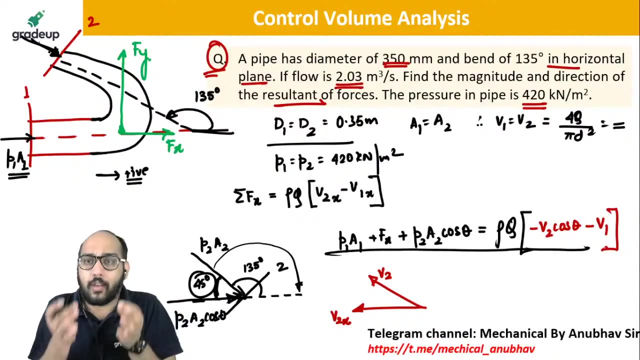 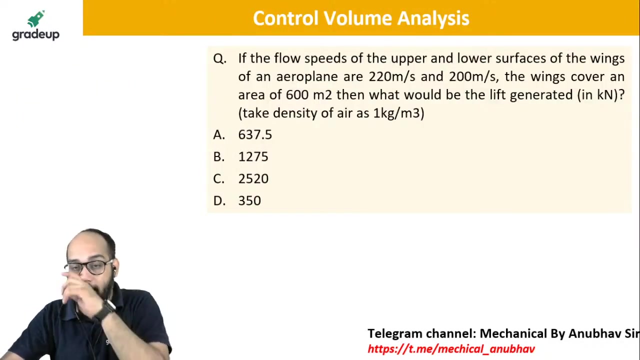 solve it. if you have a doubt, please do post it on this telegram channel. okay, so I'm moving ahead. second part, second question was just to discuss, so I do not recommend learning the formula for this case. it is better you analyze, form the equation, solve it, okay. so, moving on to some other questions and 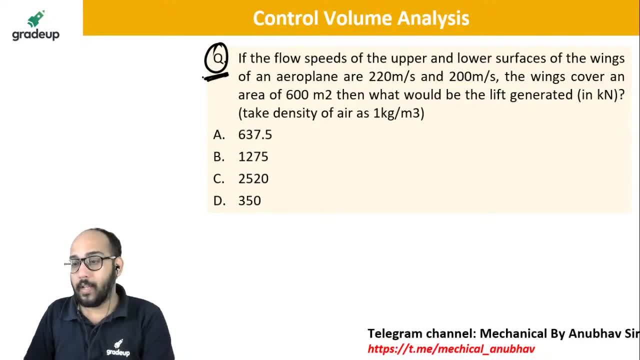 now will be a little quick. okay, these are some miscellaneous types of questions which can be asked. the first one of this category is if the flow speeds of the upper and lower surface of the wings of an airplane is 220 meters per second and 200 meters per 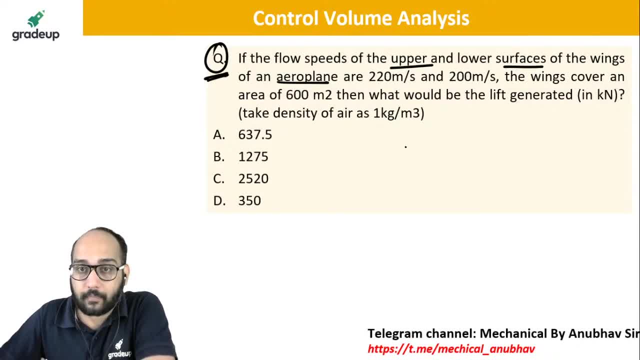 second. so there is a wing. okay then, this is the wing of an aeroplane and the top part you. this is the top part of the network. okay, haha, this is the bottom part. okay, so at top, what is the velocity here? 220 meters per second and v2, here is 200 meters per second. the wings cover an area of 600. 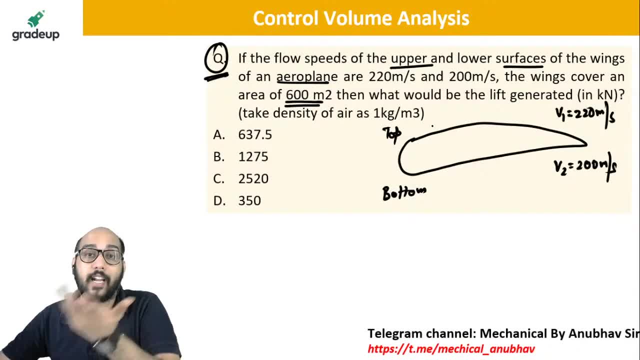 meters square, so this whole area is 600 meters per meter square. what is the lift? what would be the lift generated in kilo-meter? you can take the density of air as 1 kg per meter cube. okay, very good, very good. so the idea is: what is? 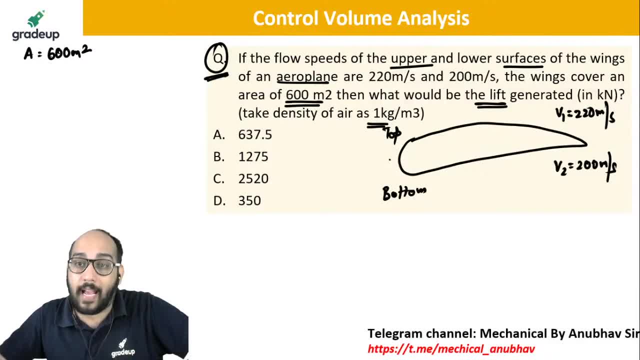 the lift. lift means what is the force that will be exerted from the bottom. from the bottom, there will be a lift. how will this force act? only when there is a pressure difference. okay, only when there is a pressure difference. because of this, a force would act. so, to calculate the force, what you need to find? what is the pressure? 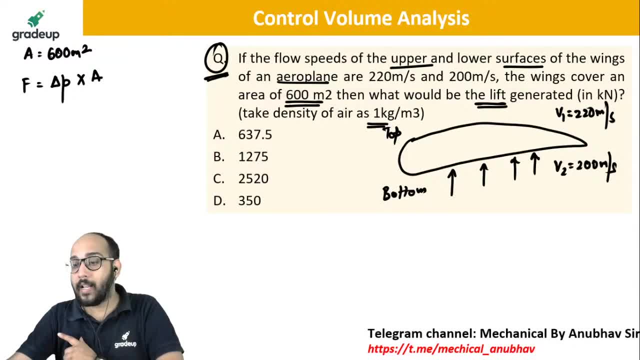 difference. multiply with by the area, you get the answer. what is the pressure difference applied? Bernoulli's equation p1 by rho g plus v1, square by 2 G plus z1, is equal to p2 by rho g plus v2 square by 2 G plus of. okay, now it is very logical if there has to be a 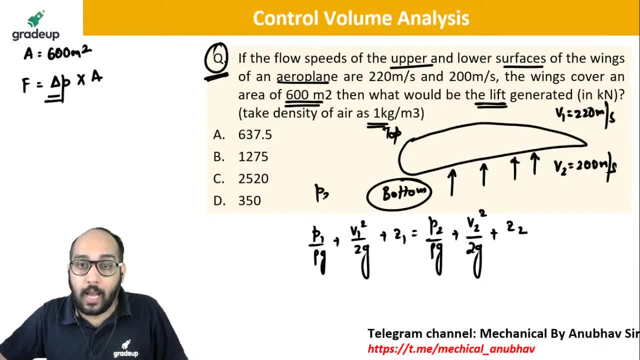 lift the bottom me to, pressure over p2 has to be greater than the pressure at p1. very logical if for a lift to happen the pressure below should be higher than the pressure up. so let me write this equation of form, this equation as p2 minus p1 by rho g. 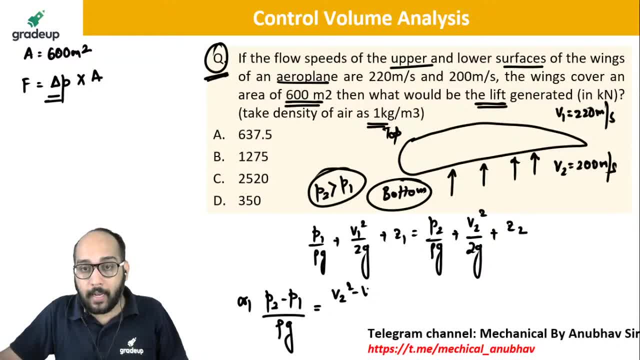 this is equal to v2 square minus v1 square by 2. G gng cancels what is p2 minus p1. it is row into v2 square minus v1 square. y2. the value of rho is 1, so v2 square is 220 square minus 200 right, divided by 2 to 6. 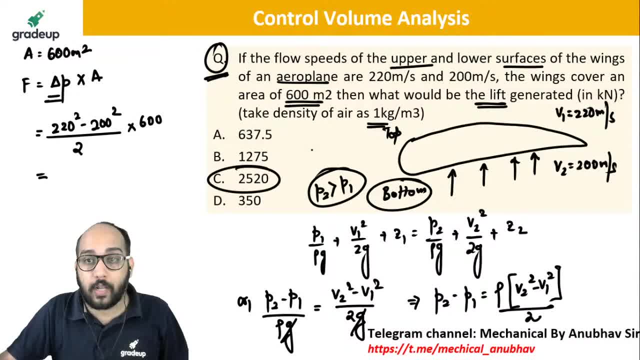 calculate this in the next video? alright, in kilo Newton. they are asking: if you solve, you get 2, 5, 2, 0 understood, just a simple application of Bernoulli's at including this, you have post calculation? okay, we doubt no, let us move to another question. you got question curry next. 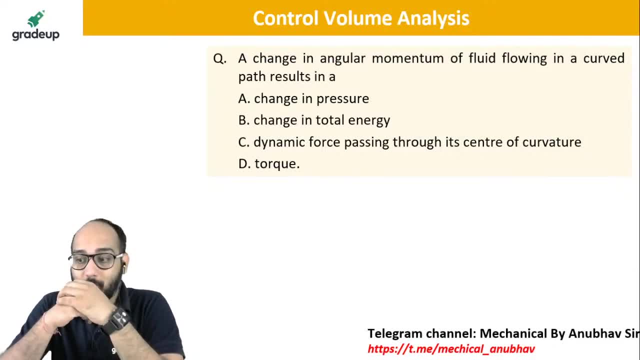 come on. a change in angular momentum of fluid flowing in a curved path results in what change in angular momentum results in? okay, so taught so what we have a beat of what we have discussed. this equation, fx is equal to rho, Q, b2 minus v1. ok, summation of fx. this is the case of when you are talking about. 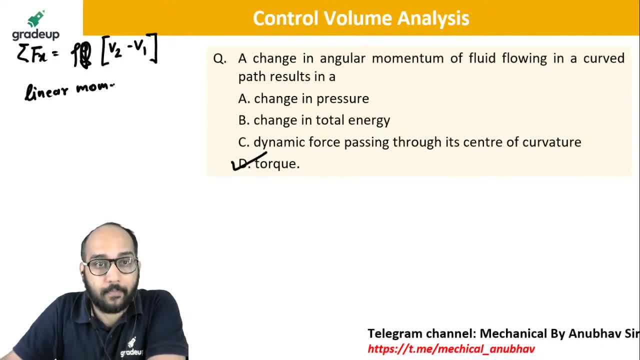 linear momentum, ok, but when we talk about angular rotating elements, what do we get? net summation of torque is equal to rho Q. now we need to have angular moment a, so it would be v2 r2 minus v1 r2. please remember this equation: v2 r2 minus v1 r1. 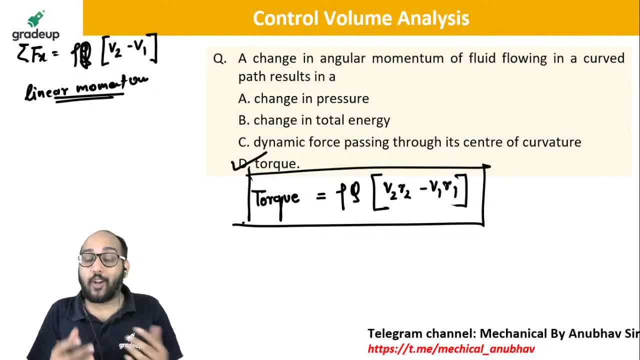 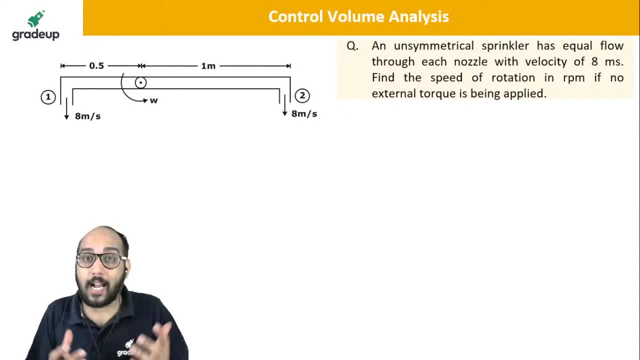 ok, and there are some additional concepts associated with it. let us try and solve one numerical, okay, so you can see that it's 1 0, 1, 0, 1. ok, Ok, understand the criticality of it. So what does it say? It says that an. 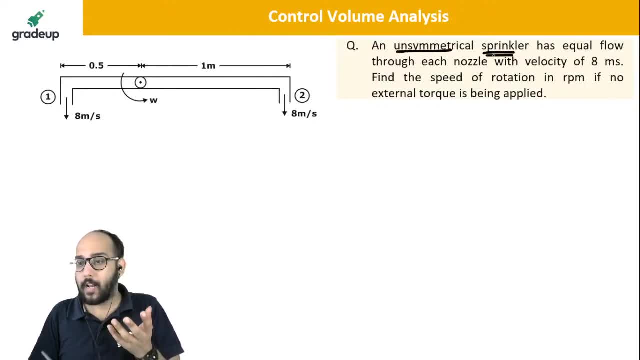 unsymmetrical sprinkler. What is a sprinkler? Anyone who plays football or watches football, football, hockey, these kind of sports? No one. Maybe in some of the sophisticated lawns gardens you see these kind of things: Sprinkler. 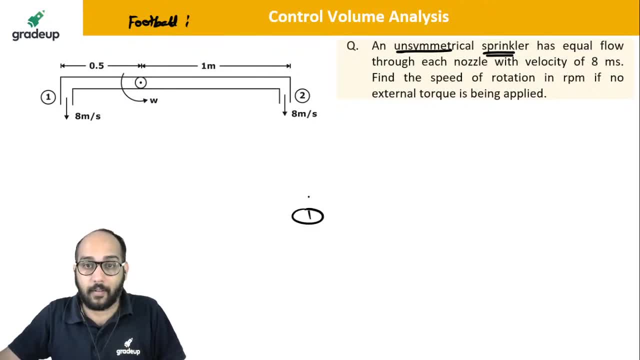 So these are kind of rods. They have nozzles mounted and they rotate, They rotate. Yeah, I definitely shared. Maybe I forgot. So you have this in the lawns which come out, and then they rotate and they are discharging water. 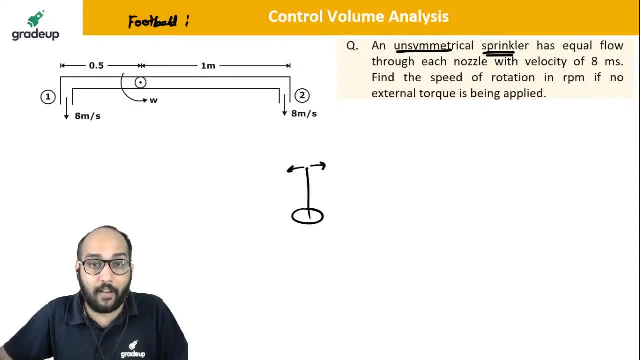 That is a sprinkler for you. So its view is given. is this? So it is unsymmetrical, not at the center. unsymmetrical Has equal flow through each nozzle with velocity 8 meters per second. Find the speed of rotation in rpm, if no external torrent. 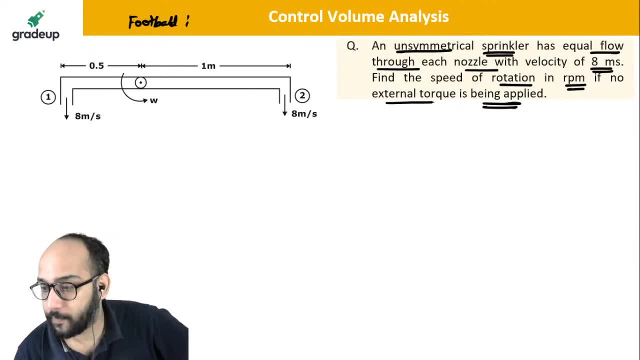 is required, Sir. the concept with v-Omega comes in hydraulic machines. We talk about whirl velocity. So v-Omega 2, u-2, all those things would come in hydraulic machines. Okay, Hi, Krishna Chaitanya, very good evening. Yes, sir, Okay. 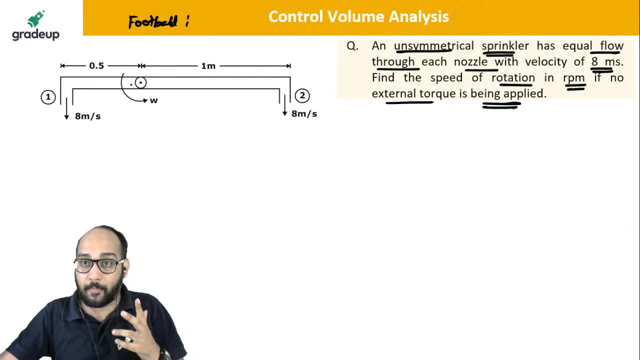 Yes, you have seen it. Okay, So this is that device, sprinkler. now this is with which 8 meters say water go, bolai. Now understand this very important point, very, very important point. This is one of the linear velocity, but not the total velocity with which water is coming. 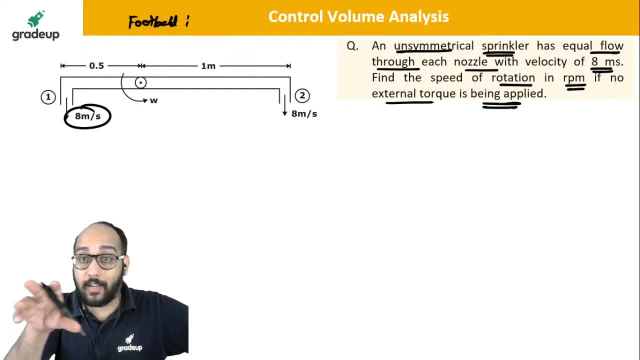 out. okay, It is not the total velocity with which water is coming out, because you need to understand if it is rotating in this direction. If it is rotating in this direction while the nozzle discharges, both of them want to discharge in this direction. 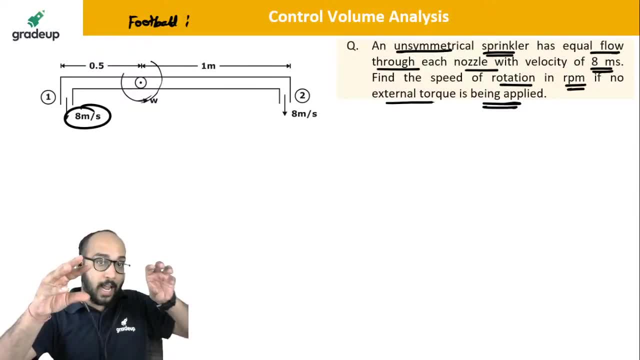 But what happens? one rotates in this direction, another represses. What happens? Will there be a relative velocity or not? Will there be a relative velocity? Both of them, ideally, if they are at 8 meters per second, so both of them will discharge. 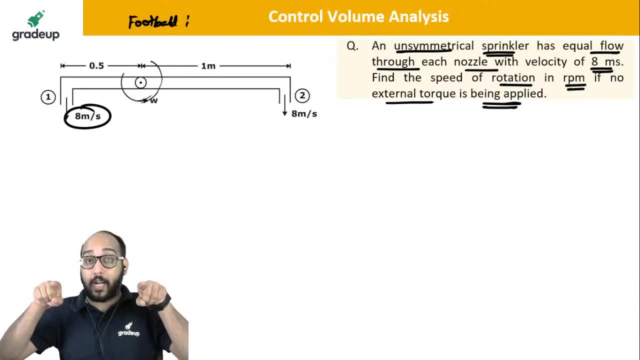 water at 8 meters per second. But what is happening? They are rotating. One goes in this direction, another is: usko aap peechhe leke aaro. there will be relative velocity, Okay, And when we add V1,, V2, all those things, that is the total velocity which we are taking. 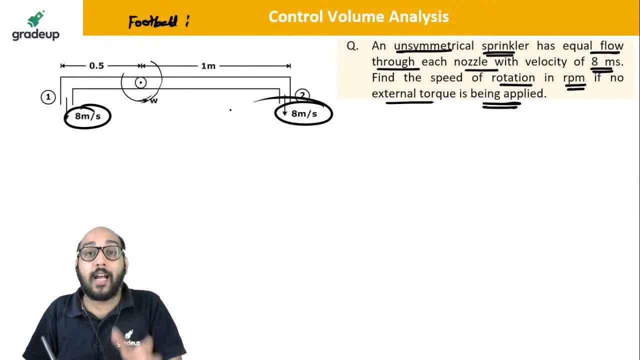 Okay, So yaha pe sabse. pehla point is That you need to add that linear velocity which is accounting because of rotation of this sprinkler. Understood this concept, Yes or no? Okay, Good, Good, Good Good. 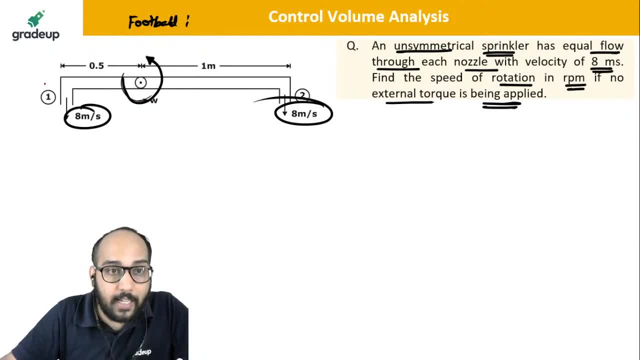 Okay, So here, whatever it is discharging because of this omega- can I say it is omega R1 or omega R2- would be in this direction. So this is section 1.. So can I write: V1 is 8 plus omega R1. 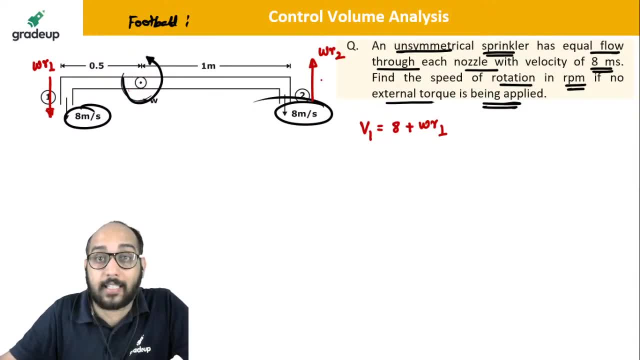 Now you would say, sir, why have you taken this in this direction, omega R2 in this direction? No, Because it the direction of rotation is given. Because of this direction of rotation, this section 1 would come forward. 2 will be going. 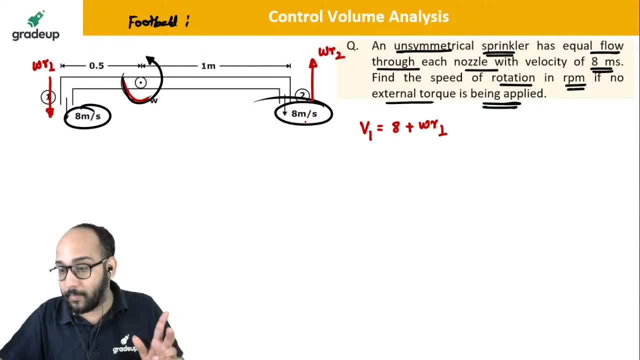 back. So that is why I have given them the direction. Okay, Now they are not at the symmetry, not at the center alaga, like this inside. So this is R1, this is R2.. I do not know what is omega. 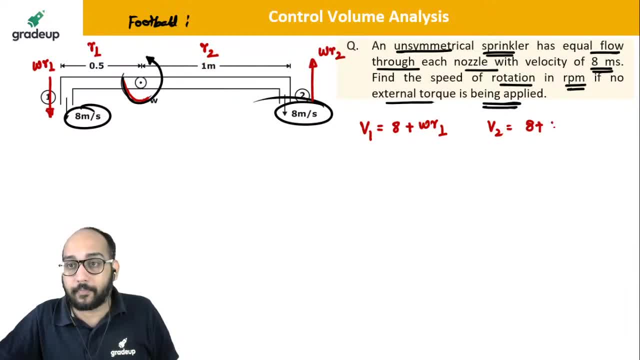 So V2 is 8 plus omega R2.. Sorry, minus omega R2.. Okay, Now they are telling me, if I write the equation torque is equal to rho into Q, V2, R2 minus V1 R1.. 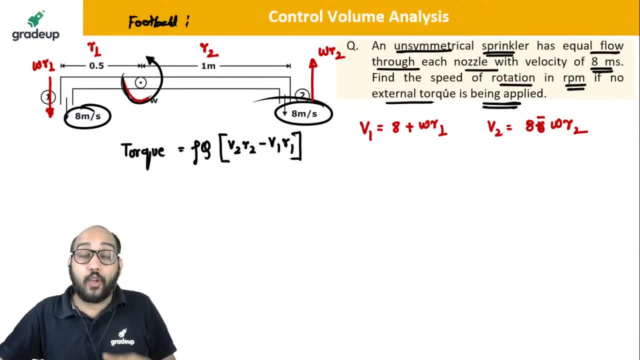 So this is valid, But they are saying that you need to find the speed of rotation so that there is no external torque. that is being applied, Okay, Okay, Okay, No external torque. Now can I write this value to be 0?? 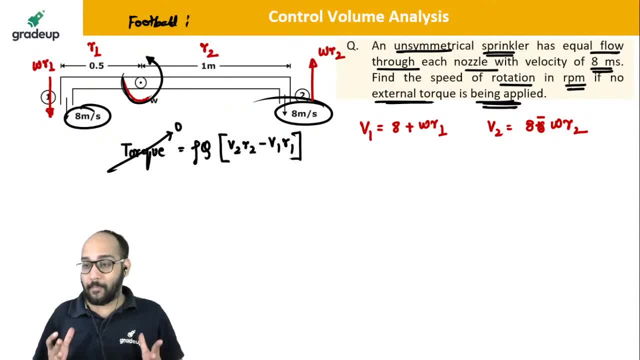 Because in the equation it is given, no external torque is to be applied. So now external torque is 0, so that value goes 0. Now this whole thing becomes equal to 0. Density value cannot be equal to 0.. 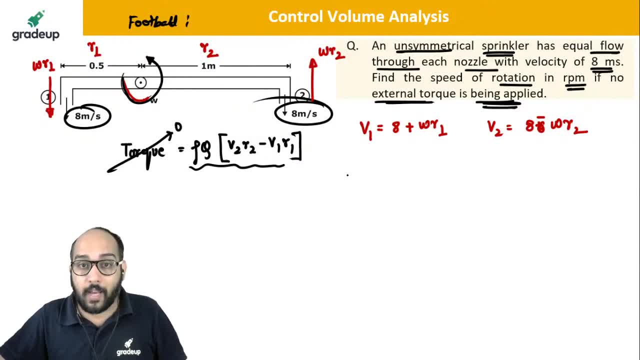 Discharge also cannot be equal to 0. So from here we can directly write: V2 R2 minus V1 R1 is equal to 0, or V2 R2 is equal to V1 R1.. Okay, Now let us put the value. 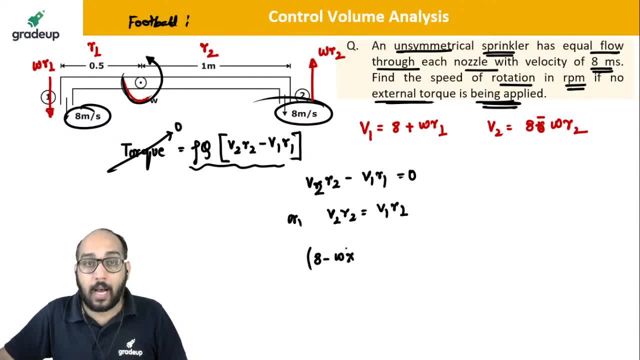 What is V2?? It is 8 minus omega. R2 value is 1 into 1 minus V1, is 8 plus omega into 0.5 into 0.5.. Okay, This is 8 minus omega. This is 4 plus 0.25 omega. 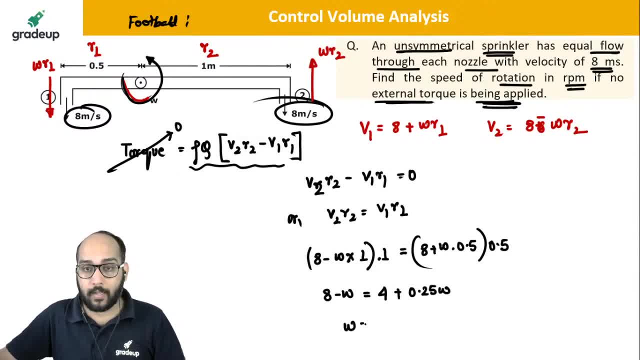 So from here, what do you get? the value of omega. So this is 4 divided by 1.25.. How much is it? This is what. 3.25, is it Okay? 3.25, is it? 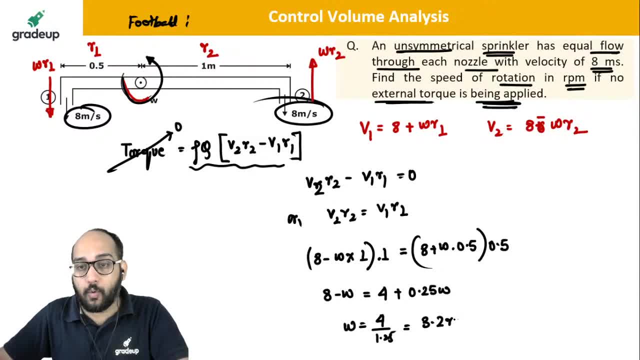 Yeah, 3.2. This is 3.2 radians per second for our answer. Fill in the blank: are 3.2 is the answer Yes or no? But, my dear friends, again small mistake. many people do asking the speed of rotation: rpm, not Omega. 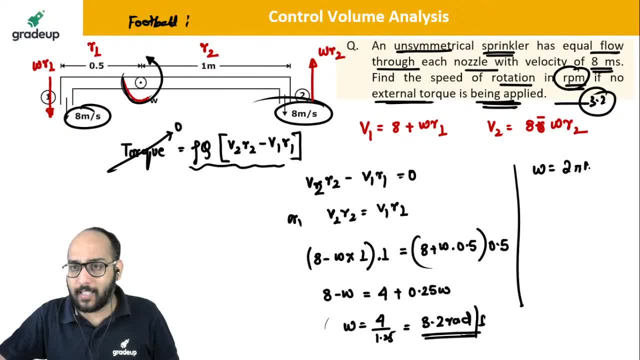 Okay, so Omega is 2 pi n by 60.. Yeah, I know, I know Smart log a guys, but yeah, when we try to kill a joke, mistake curving, Otherwise you all are awesome. So from here, calculate the value of this. This is 60 into 3.2, divided by 2 into 5. 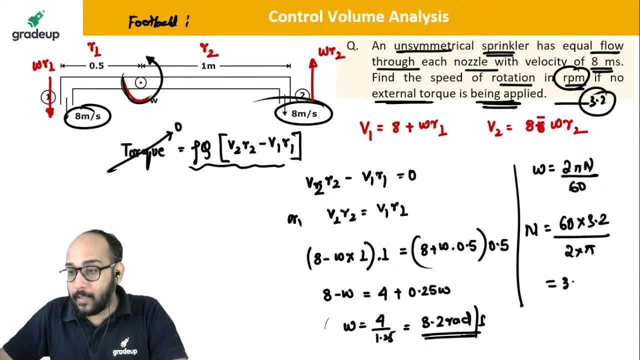 What is this answer coming as 30 point 5, 7 RTM. So We made a mistake. Okay, very beautiful question on angular momentum. you had one type, one such question in gate coming in the previous year and This type of question, believe me, is highly anticipated. 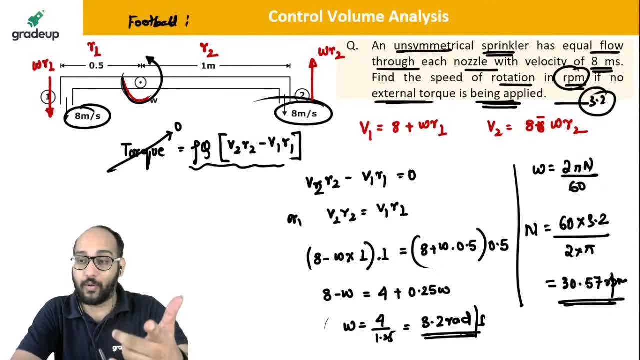 Only they're coming out of it. Oh, I got you never know. 2020 To is the lucky year, Okay, so please go through these kind of questions. This is one such. Okay, if you know the value of Omega, You can always calculate the value of torque. 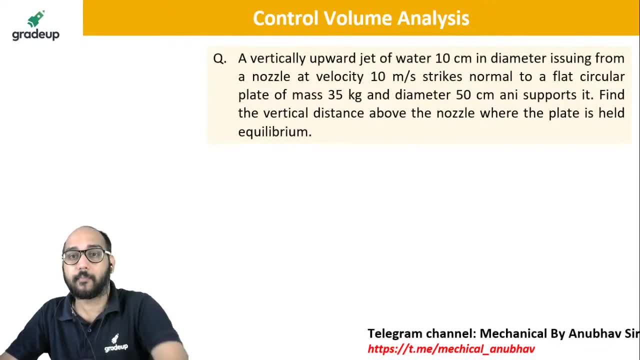 either way, okay, This is an assignment from my side. the concept is very simple. it is the concept of impact of jet, and Not only impact of jet. you can again use these principles because I want to discuss a very beautiful question: Not only impact of jet. you can again use these principles, because I want to discuss a very beautiful question. 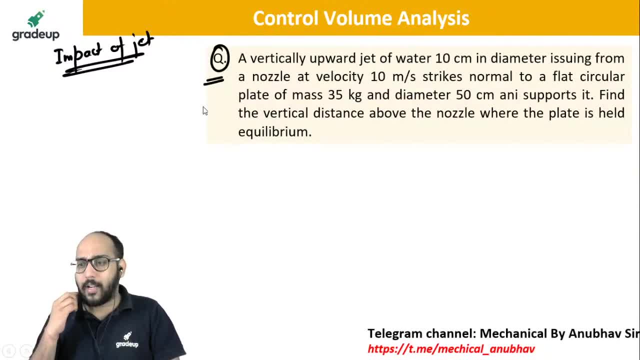 Okay, so I'll give you just the thought process. try, try this out. This is assignment from my side. Okay, Calculate the force. see a vertically upward jet of 10 centimeter Is she is coming out from the nozzle at 10 meters per second. 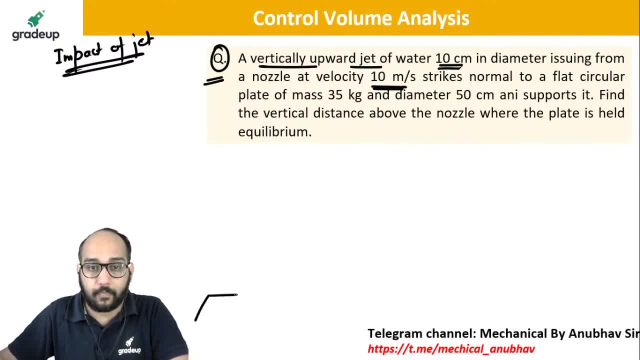 So there is a nozzle From which jet, a certain jet of water is discharged. Okay, here The velocity is 10 meters per second. Okay, Strikes normal to a flat circular plate of mass, 35 kg, diameter 50 centimeter, and suppose supports it. Find the vertical distance above the nozzle where the plate is held at equilibrium. 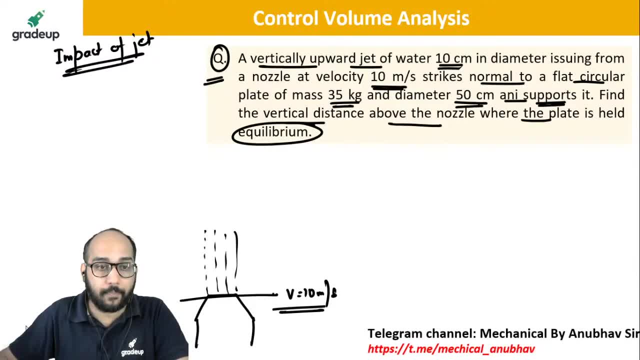 So initially say, for example, the plate was here. As soon the plate was here, if the nozzle Discharges jet of water, what will happen? they will apply some force. because of this application of force, it will take upwards and Finally it will come to an equilibrium position. So at this equilibrium position, can I write? 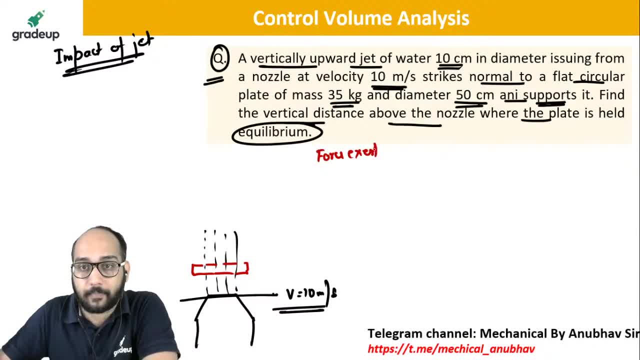 force exerted By the jet Is equal to weight of the Plate. yes or no? Force exerted by the jet is equal to weight of the plate. Okay, now for this liquid mass that is entering out. if you calculate, Fx is equal to Rho Q. 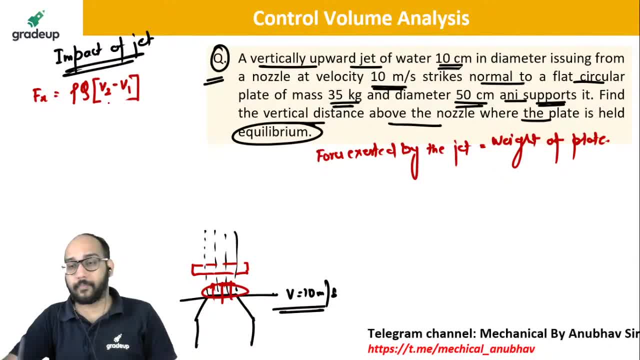 V 2 minus V 1. Okay, so ultimately this comes out to be Rho a V square. Okay, this ultimately comes out to be Rho a V square. So applying a row a V square is equal to mass into gravity. So from here you calculate the velocity with which, if the final position of the plate is here, 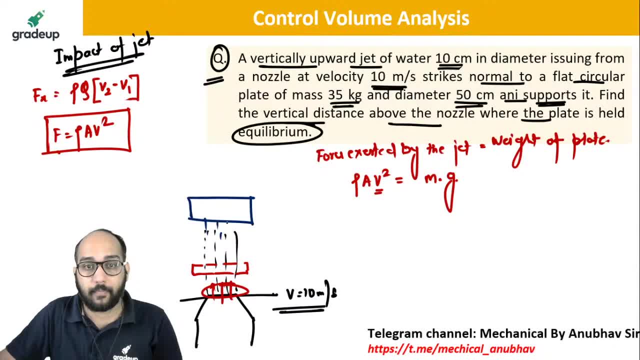 This is the equilibrium position, This is the velocity V with which it is striking here. this position, V, F you calculate. okay, then apply the basic equation of motion. basic equation of motion, What is it? V final square minus V initial square is equal to 2gh. 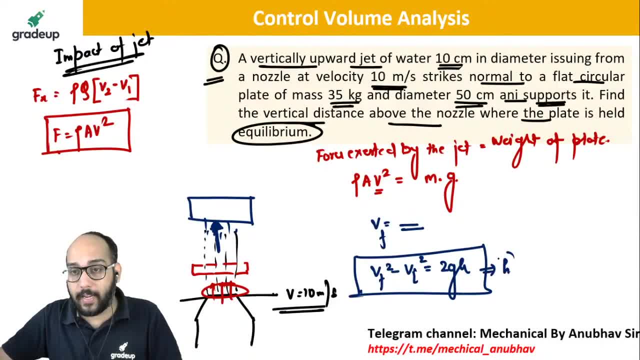 Okay, apply this, you get to calculate the value of height. Okay, so I'll just write down the value. this would be coming as 2.86 meter. Okay, this would be coming as 6.6 meters per second. Calculate this what I? because there is one very beautiful question: hai bohot chota sa. but I would like to discuss. 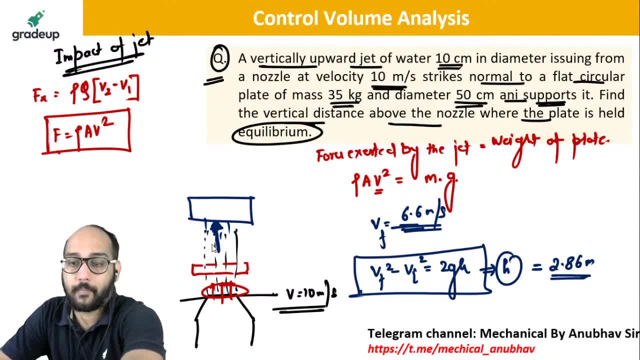 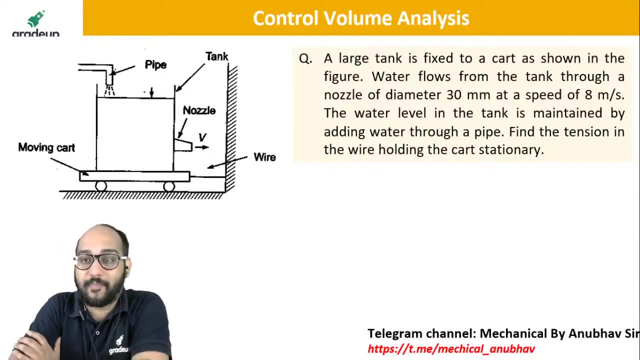 it. it is very easy. ok, this is the question, and sometimes in GATE they give these kind of questions to make you afraid. sir, pata nahi what complex diagram that they have given so much of data and you think like isko na bhi rehne dete. leave it aside, let me move. 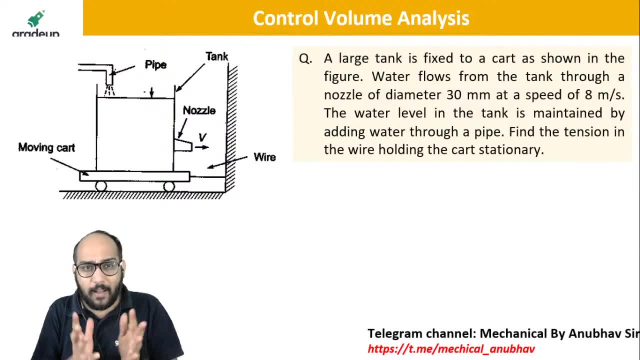 on to the next question. ok, diagram is so difficult that there is a pipe, there is a nozzle, there is a moving cart. Lars tank is fixed to a cart as shown in the figure. water flows from the tank through the nozzle 30 mm at a speed of 8 meters per second. the water level in the tank is maintained by adding water. 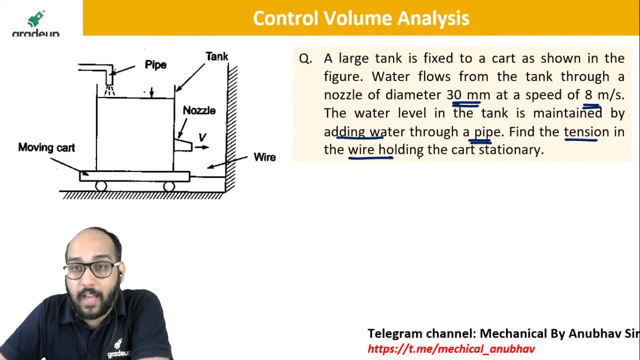 through the pipe, find the tension in the wire to hold the cart stationary at this position. yeah, water level is maintained. they have already given water level is maintained. so what is the tension that is there in the wire to hold this cart in this position? huh, only the tension. so how do we go about it? so, see, understand, if water is discharging through. 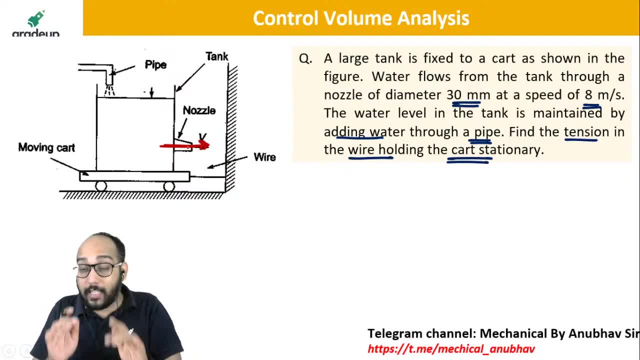 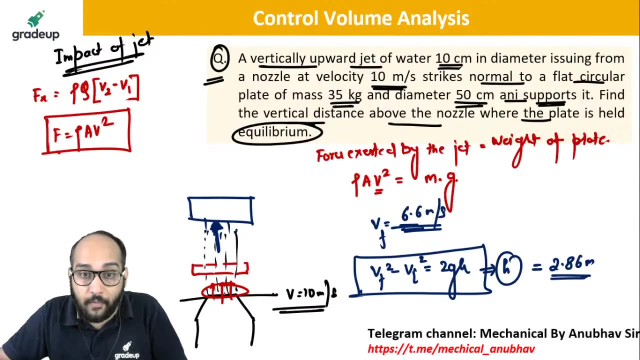 the nozzle. if the water is discharging through the nozzle, it is coming out with a force, yes or no? if water is being discharged from the nozzle, it is coming out with a force. we have just discussed this question. when water comes out, the liquid comes out from a nozzle. it can't. 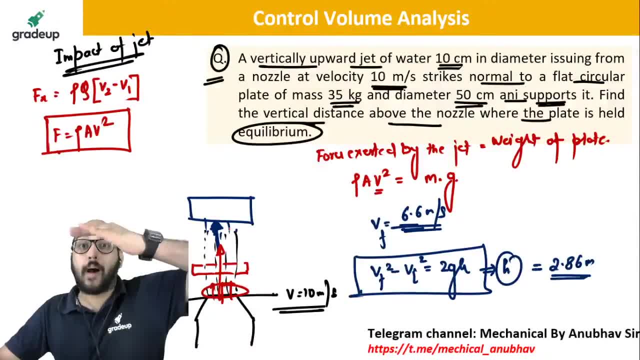 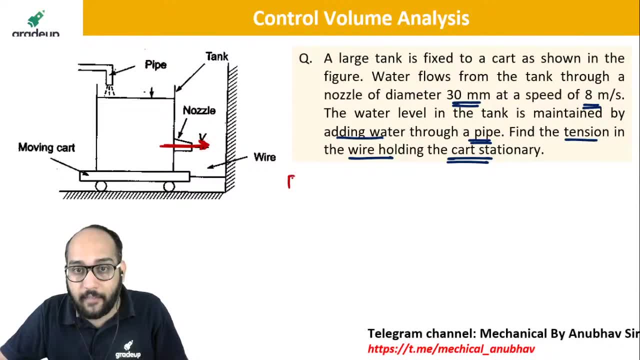 carry a force. or we have seen this: it takes this plate upwards, it carries a force. okay, so let us first calculate this force. this is in this direction: fx. this is what rho a v square. okay, ultimately why? because when it comes inside, this final velocity would be zero, because this is fixed. so rho a v square. this is 10 to the power, 3 pi by 4. 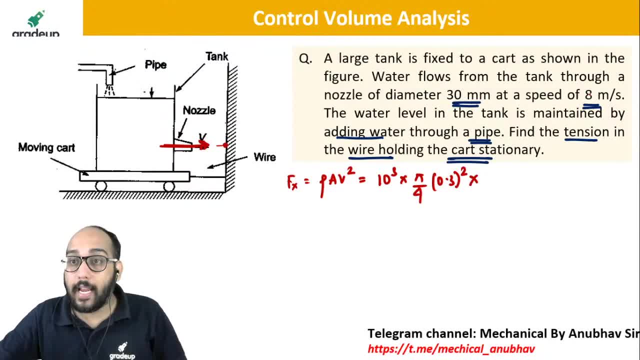 0.3 square into 8 meters per second. so could you tell me what is the force that is with this, with which it is coming out? 45.23 newton, very good scrubbing. so this is coming out with a force of 45.23 or the liquid jet can apply a force of 45.23. okay, yeah, now. 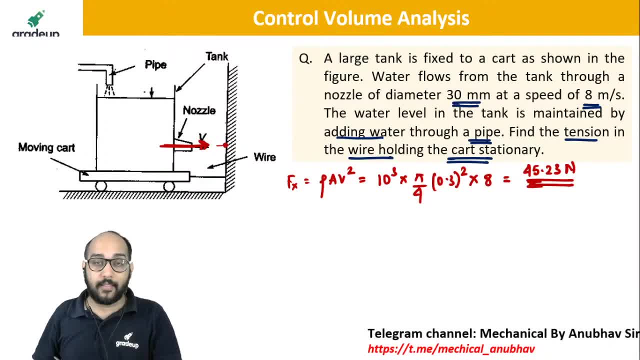 so for this goal. in case you want to see what this direction will look like now, let me explain it. so first tell me what we have seen, so now we can compute the North Sea. We high 이유 free or be jeden general climate temperature, still weather. 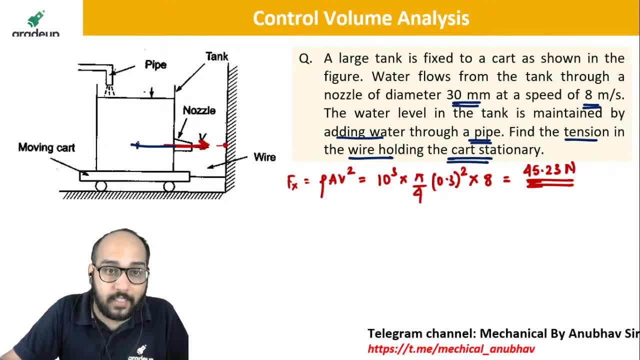 The reaction would be in which direction? This direction Equal and opposite reaction. So, because of this reaction force, because of this reaction force, the reaction would be what? 45.23.. This which direction It is taking the cart in this direction. 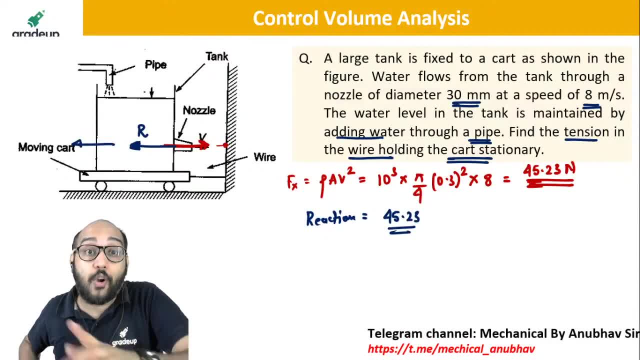 Okay, but you don't want the cart to move, So we have attached a wire here. So it is trying to move here. What is the force that is being applied to pull this? Okay square? Yes, 45.23 is coming. I have been told this answer. This is 8 square. Do I need to calculate? 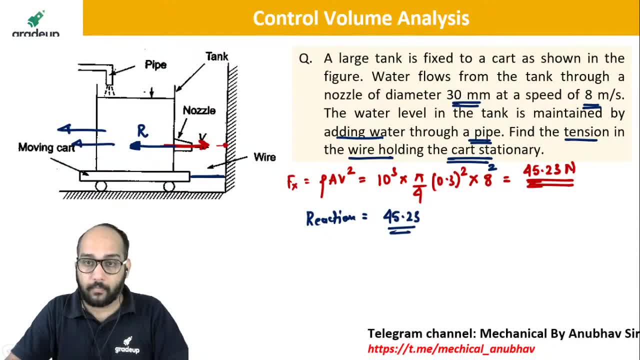 I have been told this answer: This is 8 square. Do I need to calculate? Yeah, it is coming, 4.52.. Okay, 30 mm. Sorry, sorry, sorry, sorry, sorry. This would be 0.03 square. 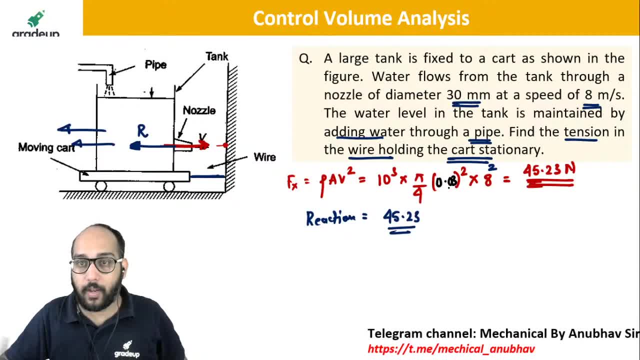 Okay, Praveen was saying this: only 0.03 square, 30 mm. Yeah, 45.23.. Correct, Okay, So reaction is 45.23.. So this cart is being pulled with 45.23.. 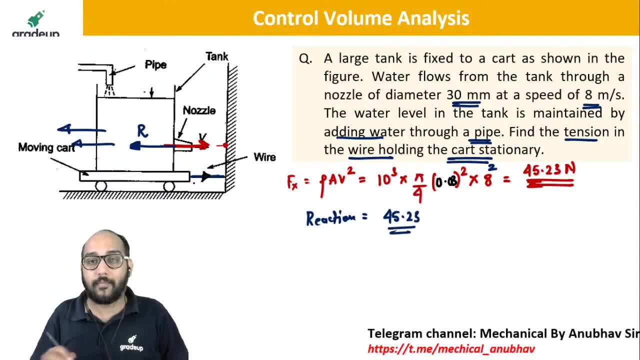 You want to keep it stationary? What would be the tension? No, no, you have done very well. My mom will also shout now. She will be shouting now, Okay, So very beautiful question. Just at the look of it, it is kind of by the look of it, it is complicated. 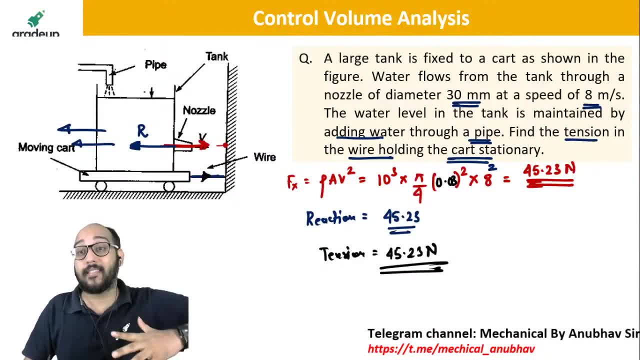 Data also seems like competitive, maintaining same head and all those stuff. But look at this question. It is just single line question, but concept is very, at a very high level. So it is that gate question which requires more of your conceptual knowledge than problem solving skills. 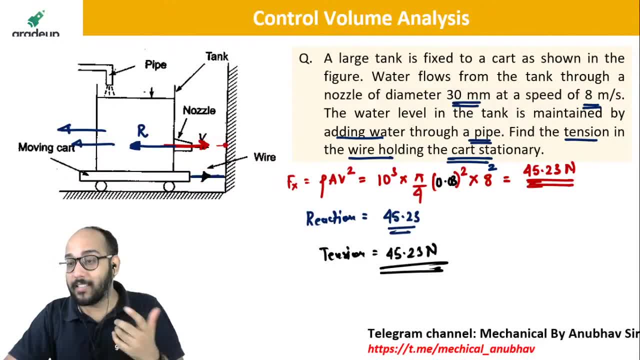 Tension. how does it come in stress? Tension is nothing but force. So it will be Newton: Tension is not stress, Tension is Your tension and your stress can be same, But here tension is nothing but force. 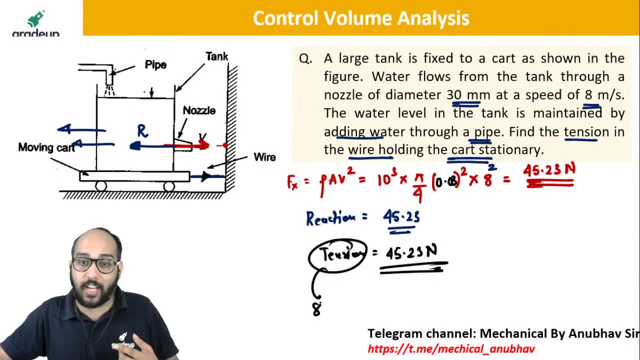 Even for us, tension creates stress. They are not same. Tension will create stress. Okay, Understood UJ styles. Okay, guys. So these are a few questions on control volume analysis. Majorly though, Impulse momentum principle, discuss karna tha. 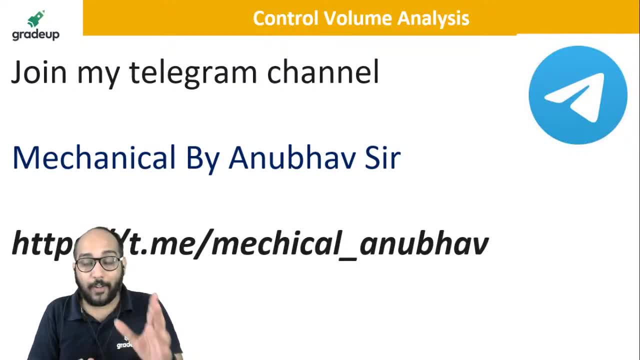 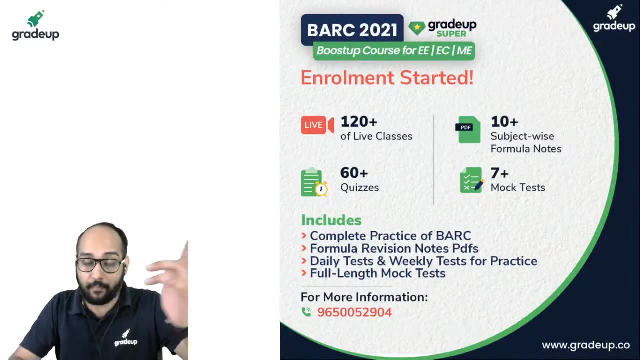 That was the important part, But apart from that, we talked about that angular momentum And then this another thing which is sometimes asked in the exams also. Okay, So these were few questions. What we have already covered are- I hope many of you are doing it regularly- 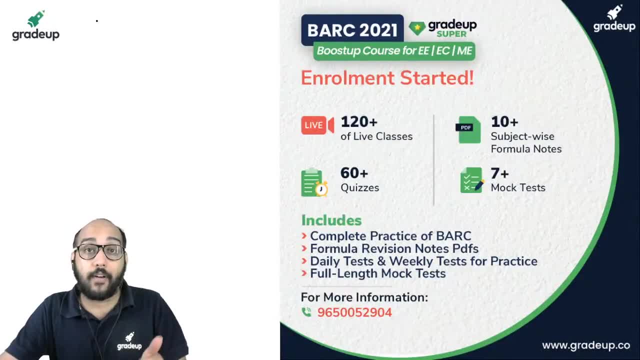 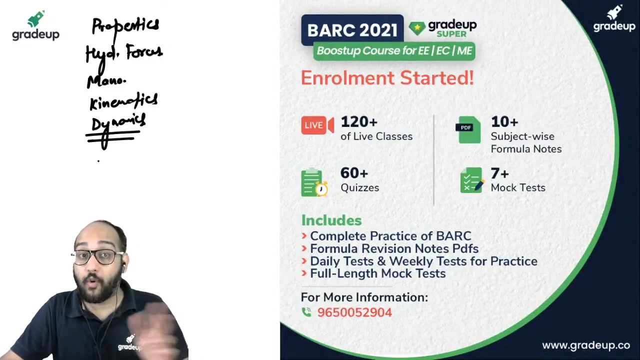 But if any one of you have missed out, we have already covered fluid properties, Manometry, hydrostatic forces, Manometry and buoyancy. We have then discussed what kinematics, Dynamics, Then measurement, Venturi orifice, So flow measurement. 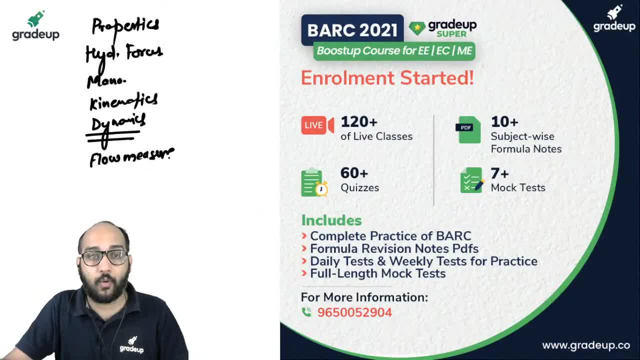 And today We have discussed about control volume analysis. So major part is this We have covered Now. from tomorrow we will move to a really important part, which is laminar flow. turbulent flow Then move on to head losses in pipes and on and on. 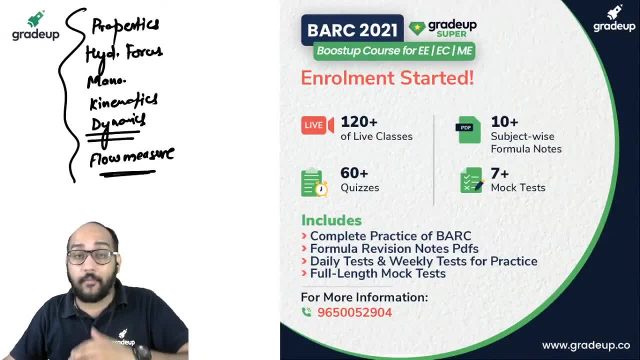 Okay, So this is what we have covered. If any one of you have missed out, these sessions recordings are available on the YouTube. Please go through it. Also, we have just launched a bar test. This is the bar course batch, which is boost up course. 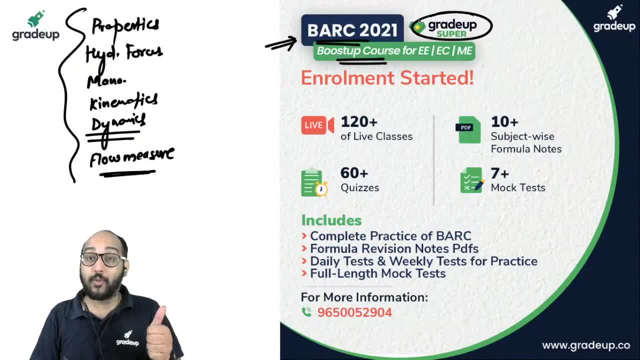 You have to have data super subscription for the enrollment. There we are discussing some questions in our live classes. Through this you get to revise your concepts. Apart from that, we will get notes, get to appear mock test which is of bark level. 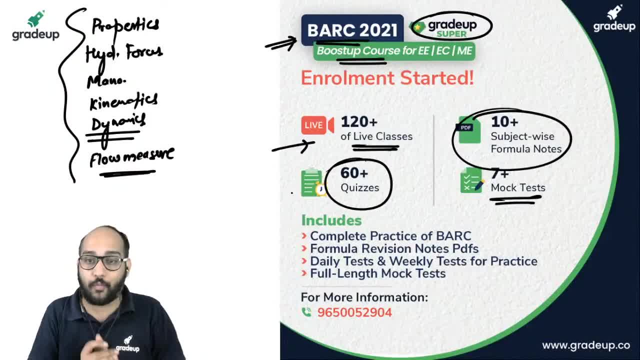 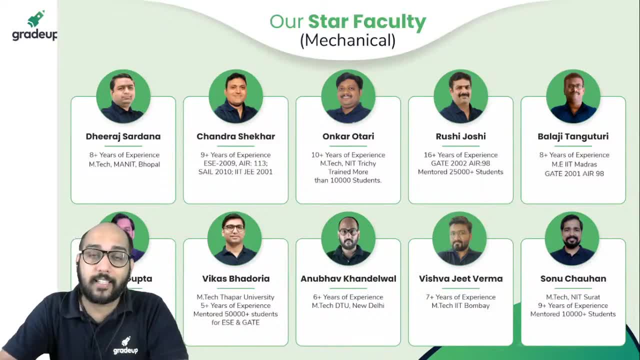 And also get to practice lot of courses. Okay, So this was all about today's session. Many other faculties like me Are taking their sessions either on the app or YouTube, So please do join their classes as well, Okay.